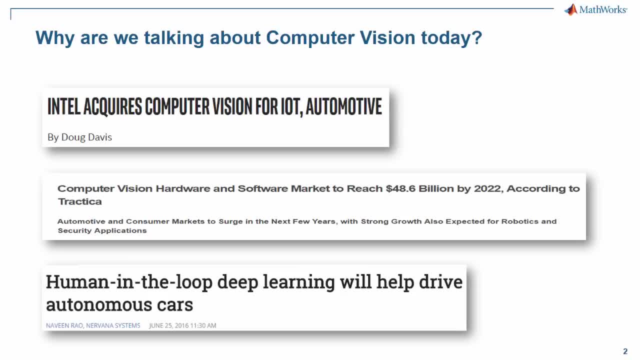 a blog, so in that blog it has been written that it's very easy to design these self-driving cars which are 99% accurate. It's very, very difficult to increase that accuracy to 99.999%, And that's very necessary because when you're traveling at a speed of 100 miles an hour, 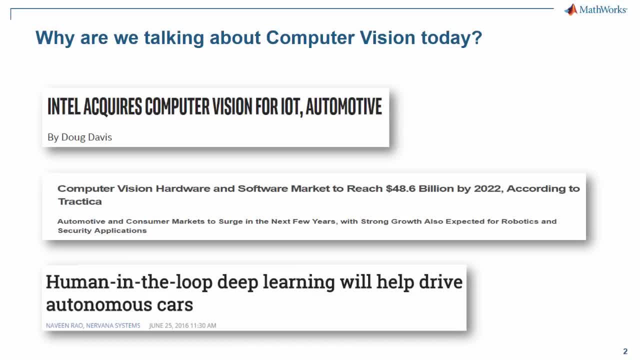 100 kilometers an hour. you just can't afford to make any mistakes. Mistakes are going to get disastrous then. So for those purposes, you know computer vision is and deep learning go hand in hand. So if you want to design something for collision avoidance or driver, 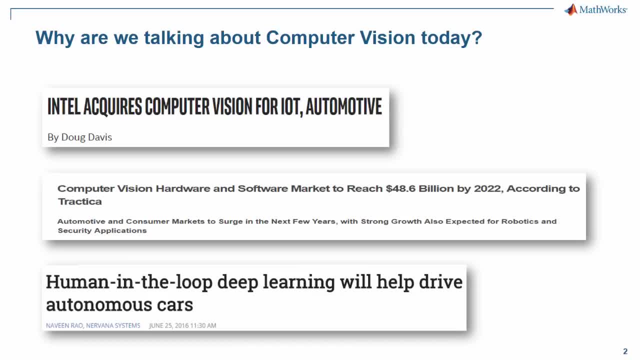 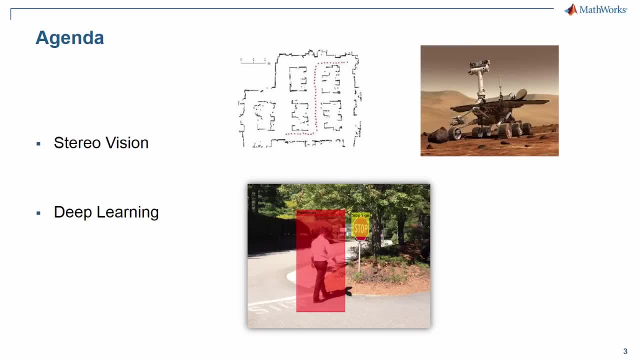 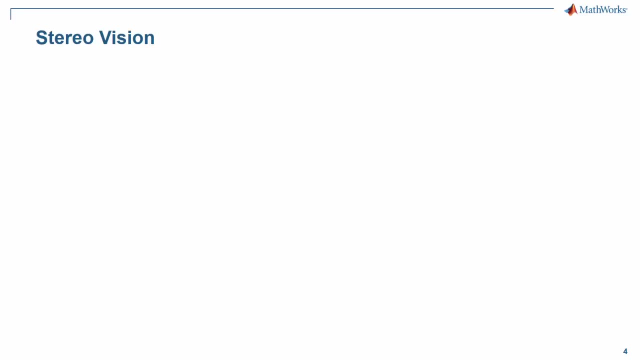 assistance systems. that's where deep learning and computer vision is important. So let's focus our agenda on these two topics: 3D or stereo vision and deep learning. So let's start with stereo vision. What is stereo vision? The stereo vision is the process of 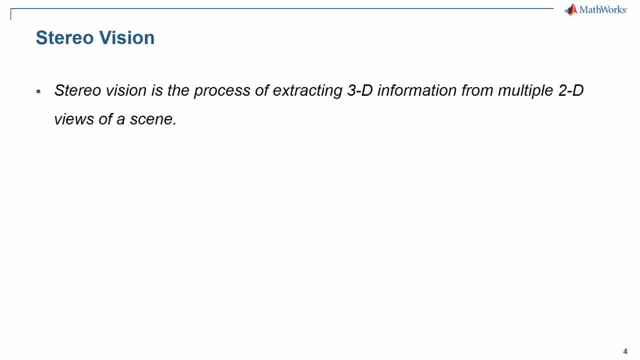 extracting 3D information from multiple 2D views of a scene, And in a while, though, I've got with me two cameras which are trying to get multiple views of a 2D of a 2D scene. So I've got two cameras with me. I'll be showing you that in a minute. So stereo vision is. 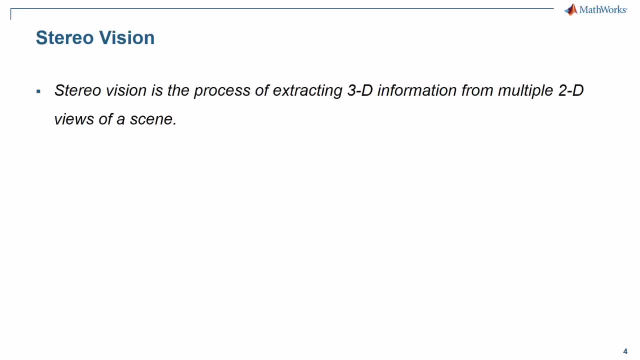 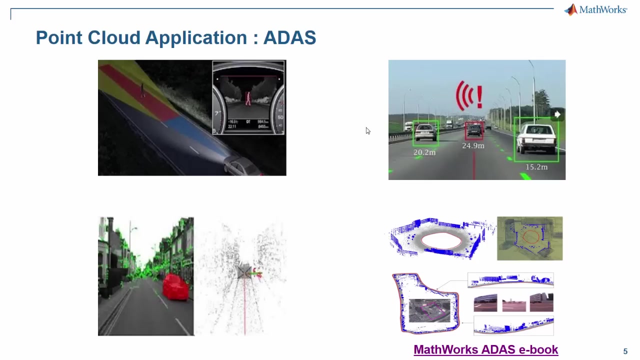 there any MATLAB product which will help me do that? Yes, there is. And the computer vision system toolbox. This just has those capabilities to do the 3D point cloud. And this point cloud application is heavily used in ADAS systems: collision avoidance, collision detection odometry. 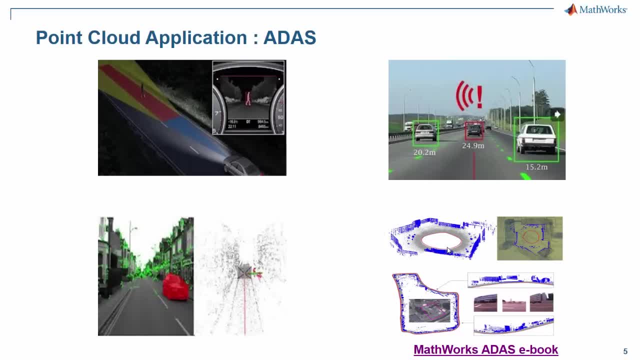 If you want to. if you're surveying a geographical region, you want to understand the area of the geographical region. Is it possible through odometry and point cloud application? This is There's over here in this particular slide. I've also introduced a link to a MathWorks. 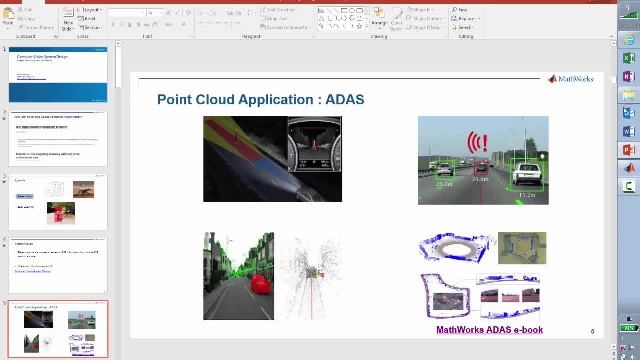 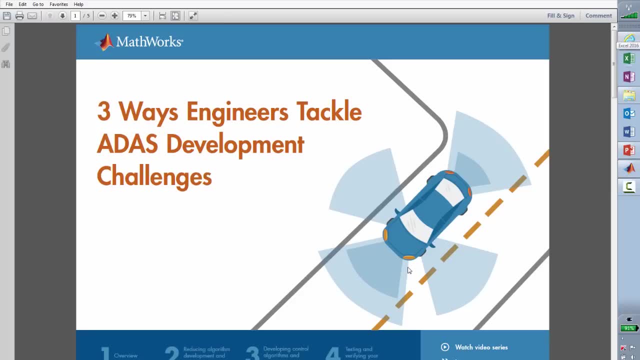 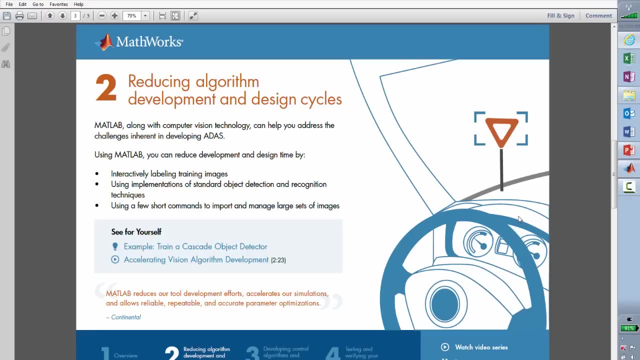 ebook on ADAS And that ebook talks about the different challenges and how MathWorks can help you overcome those. So this particular ebook is giving you an overview, some examples, some videos and how and some quotes from these famous companies of how they have used 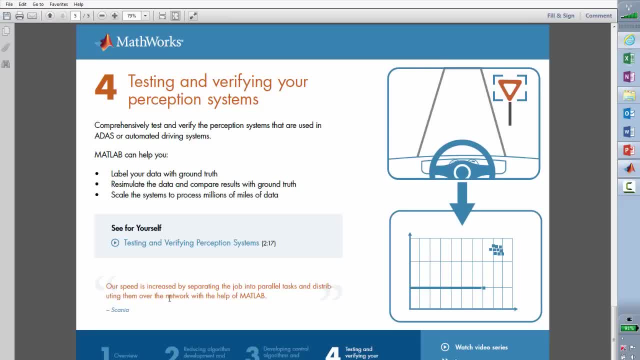 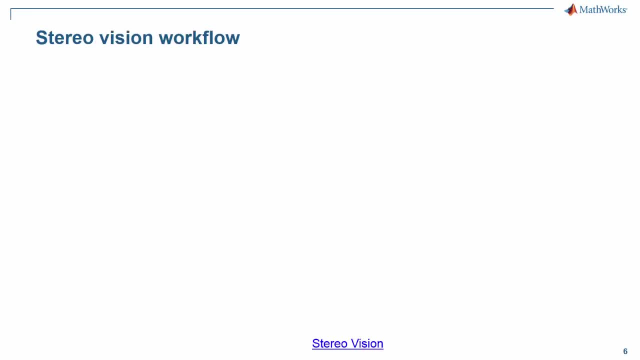 uh, Matt works products in their specific application. Okay, So what does studio vision? so we having seen what studio vision is, how can MATLAB help me get those 3D information from multiple views of a 2D scene? So over here, in this particular slide, I have introduced a workflow, So we are just using 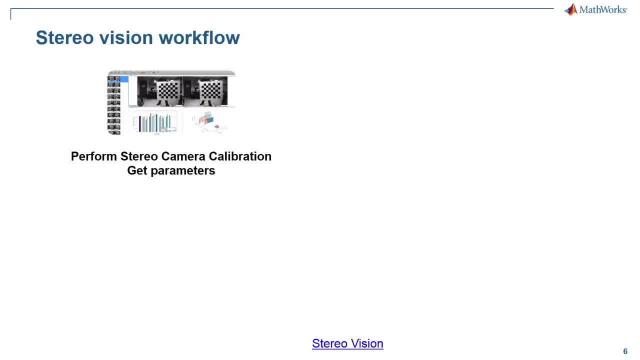 regular cameras. I've got to logitech cameras with me And to start with Studio Vision. the very first step is to calibrate the camera. If your cameras have already been calibrated, you can totally skip that step. But let's see how MATLAB can help you calibrate the cameras. 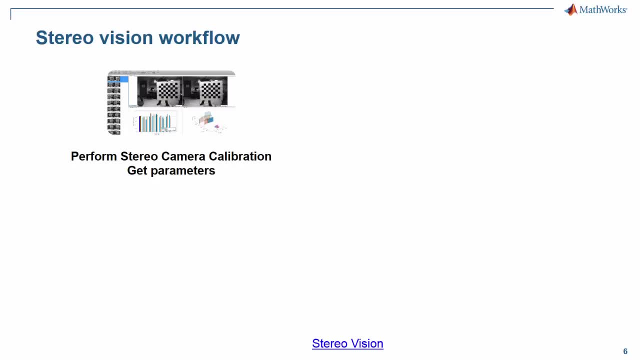 And once you calibrate those cameras, you need to get some parameters- how one camera is looking at a particular object with respect to the other. So those parameters need to be extracted. And once you extract those parameters, once the camera is calibrated, 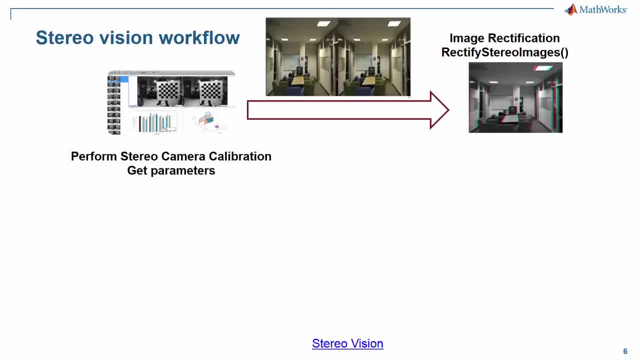 start the live acquisition of the scene, apply those parameters to the scene and rectify for any errors. So that's the second step if you want to go for going towards Studio Vision Once you distort or undistort those images by applying those parameters. 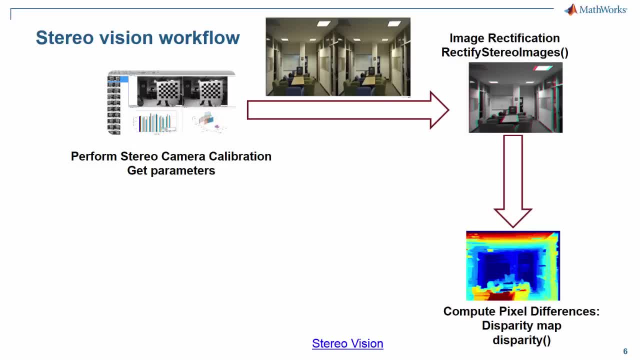 you want to calculate something called as a disparity map or the pixel differences. So what's the difference between the views of those cameras to a specific object? That's a disparity map. And once you have the disparity map, you need to put everything together to design this 3D Point Cloud. 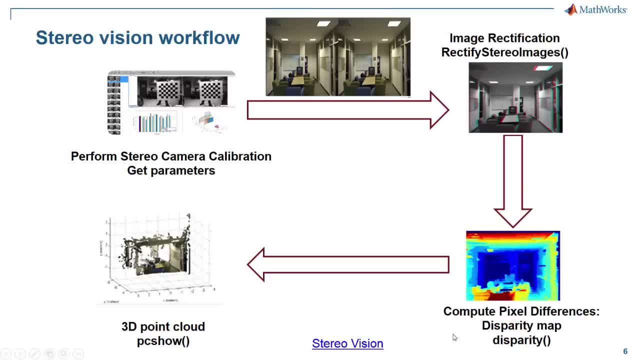 Over here in this particular slide you will also see these function names: Rectify, Studio Images, Disparity Map, PCShow and so on. So these function names are called a disparity map. So these function names are called a disparity map are a part of the computer vision system toolbox. 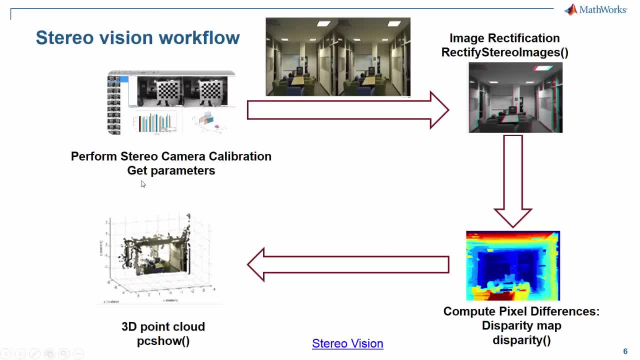 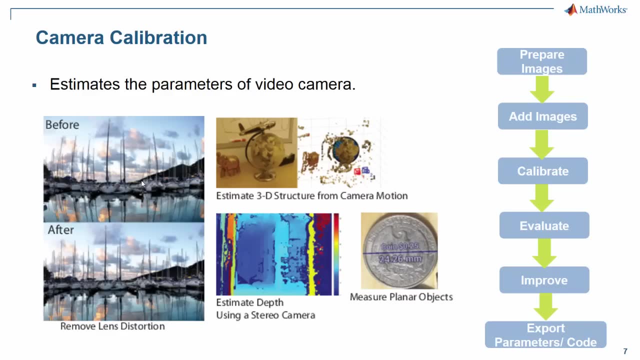 However, I haven't given any name of a function to the first part, the first step, which is a camera calibration. There's a reason for that And we'll see what that reason is: Camera calibration: you need to estimate the parameters. 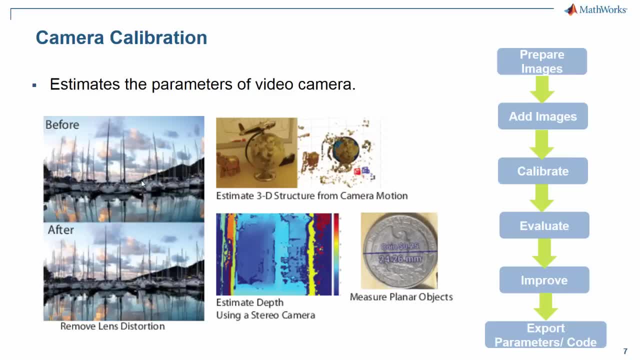 of a video camera For various reasons. you may want to remove some lens distortion, You may want to estimate a 3D structure, You may want to estimate depth, Or you may want to measure some objects. And on the right hand side over here on this slide, 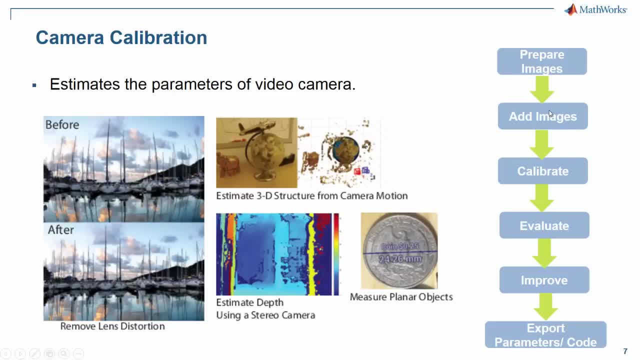 I have given the workflow of camera calibration. So prepare images, add those images. Once the images are added, calibrate them, Evaluate for their accuracy. If the accuracy is not sufficient, improve the accuracy And, once the accuracy is sufficient to your needs. 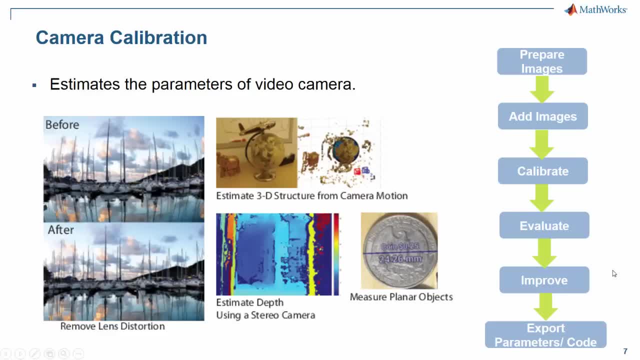 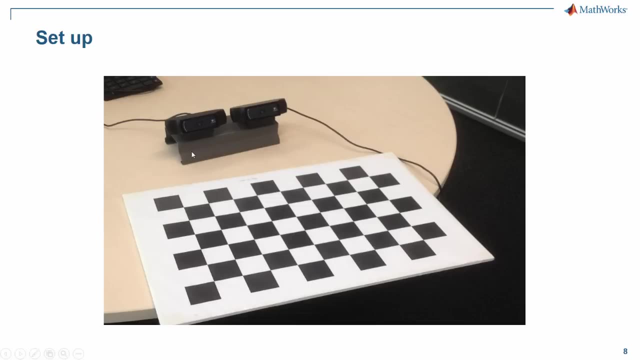 you can export The parameters. Now, what is this with respect to Where to add those images, How to calibrate the camera? So let's have a look into all those things. So that's the setup I have. I have got two cameras, Logitech cameras, mounted on a post. 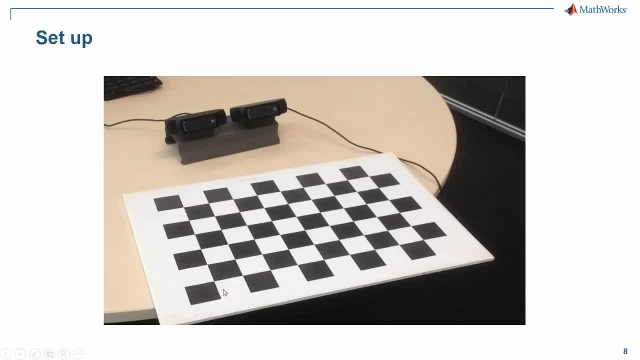 And I've got the checkerboard with me And the checkerboard is a great tool for calibration. Both of these cameras are connected to the computer, to the USB, through a USB cable, So they are connected to the computer so that I can use them. 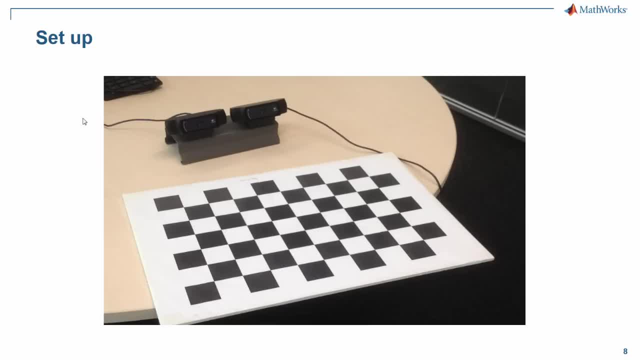 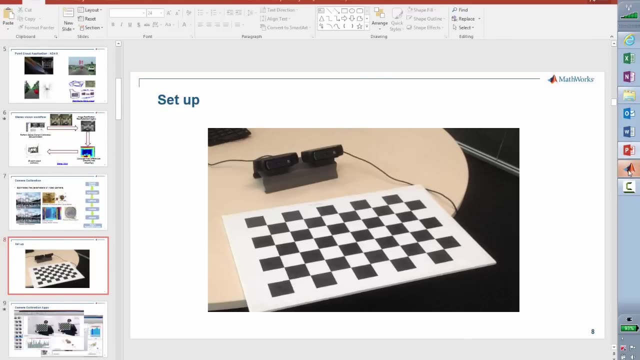 I can use MATLAB to control them. OK, So once these cameras are tied to my computers through the USB cables, let's try to file them And let's try to acquire some images. OK, So over here I'm into my folder. 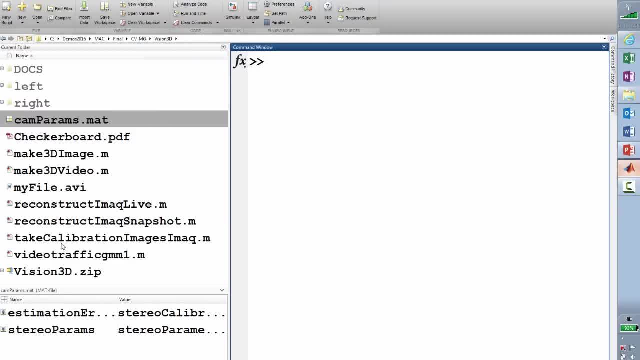 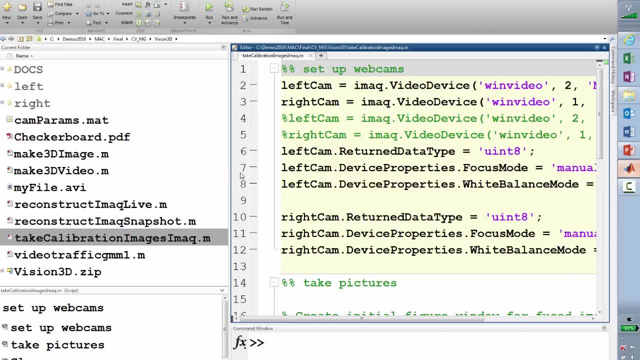 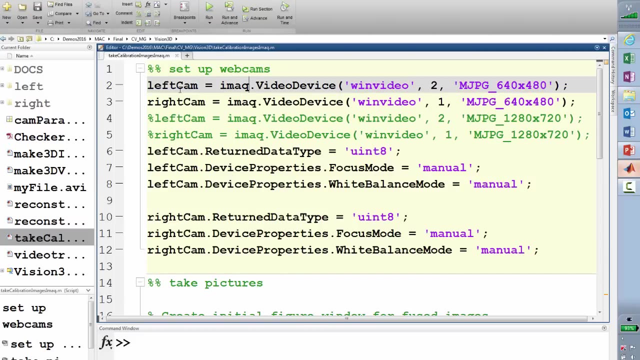 I'm going to start with acquiring images for calibration. So take calibration images. How can I start these cameras And how can I start acquiring these images? So over here I've got two webcams, the left and the right one. I'm just initializing them. 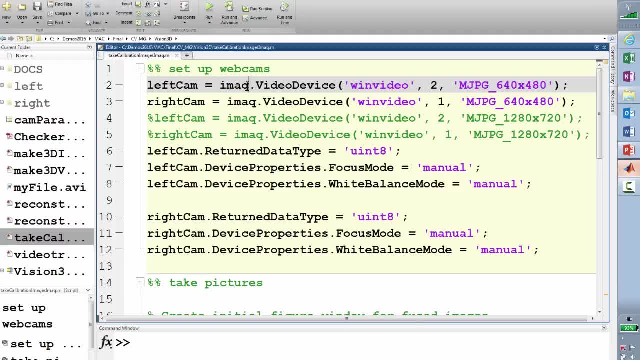 So iMacvideoDevice, VideoDevice, VideoDevice- This is the image acquisition toolbox function, And then I'm just setting some parameters. How do I want to acquire those images? I want to acquire them in unsung images, aDataType and so on. 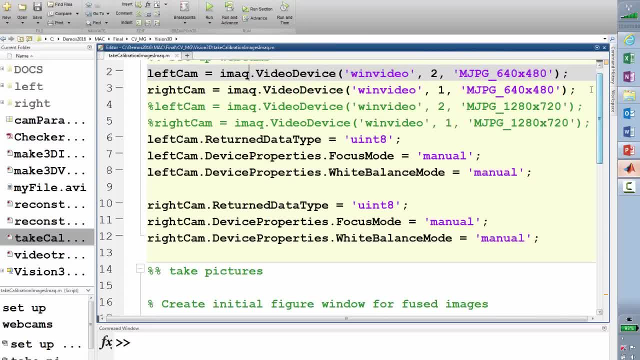 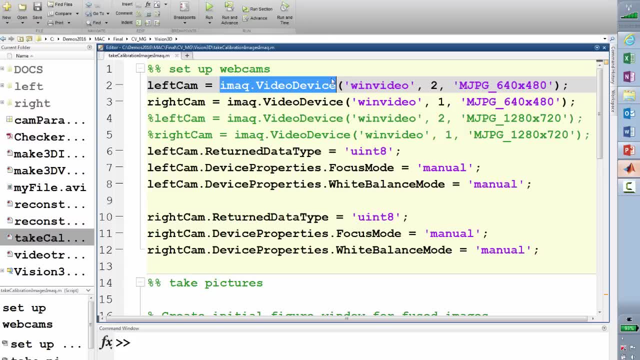 So that's the setup, And once it has been set now, what this is called is the system object. This is just setting up the cameras, And once you want to use the system object, all you'll be doing is materially. it's really just a simple setup. 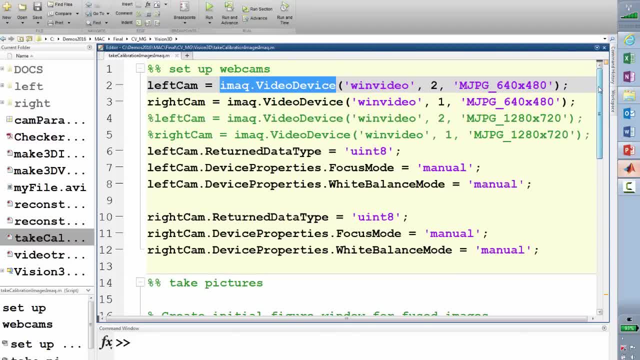 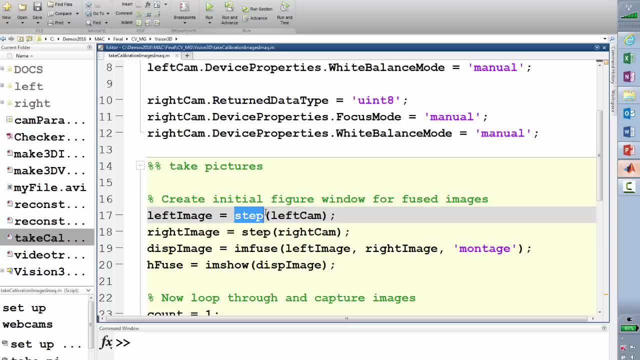 Let's just go ahead and set up the cameras, OK, OK, OK, OK, OK, making use of the step function. so left cam and right cam. so if you want to start fire up the left cam and right cam, all I'm doing is using the step function. 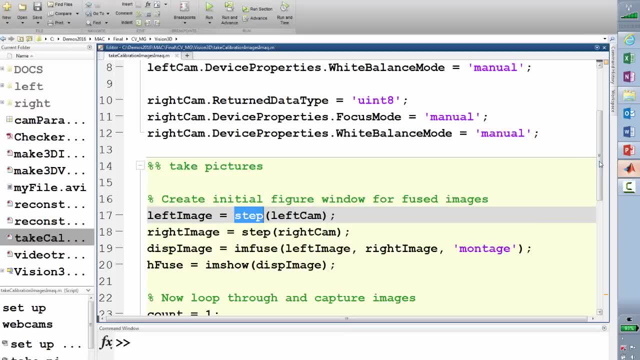 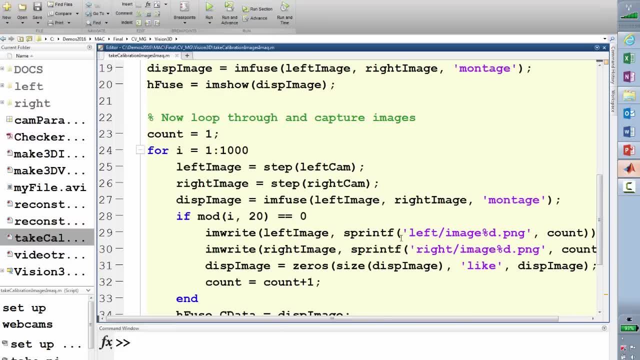 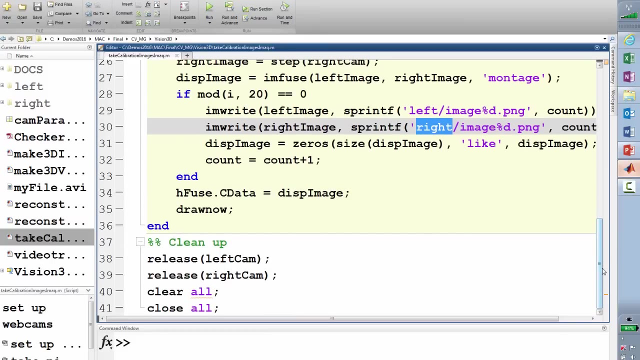 and once the step step function is used, I'm taking 50 such images and I'm writing these images to the respective folder. so left images from the left cam are written in a left folder. images from the right cam are written into the right folder. so I won't be taking images now. I've already done that. I have ran that. 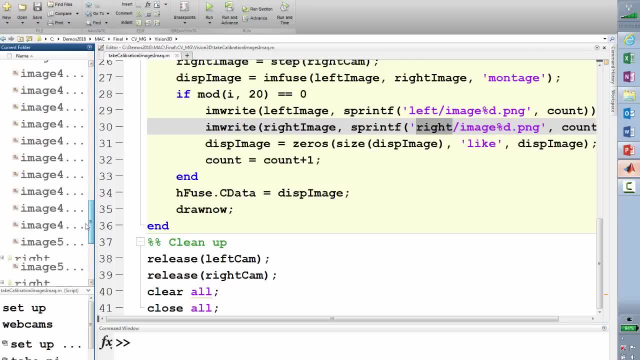 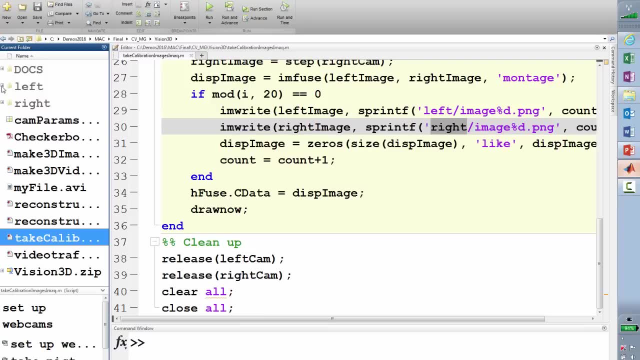 script and I've got 50 images in the left folder and I've got 50 such images on the in the right folder. now let's try to see how can we calibrate the camera? how can we obtain those parameters? now for calibration purposes? you need to. 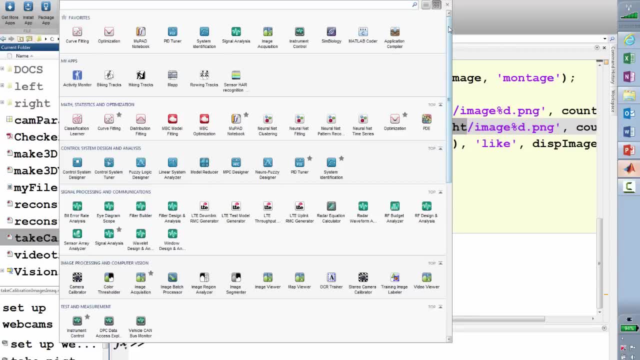 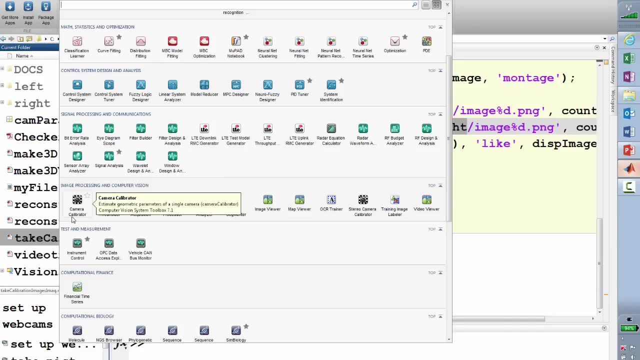 evaluate all the images on the left cam and on the right cam and then calibrate. visit the Apps tab. In the Apps tab you have, if you go under Image Processing and Computer Vision, you see those two camera calibrator apps: The one with the camera calibrator, that particular app. 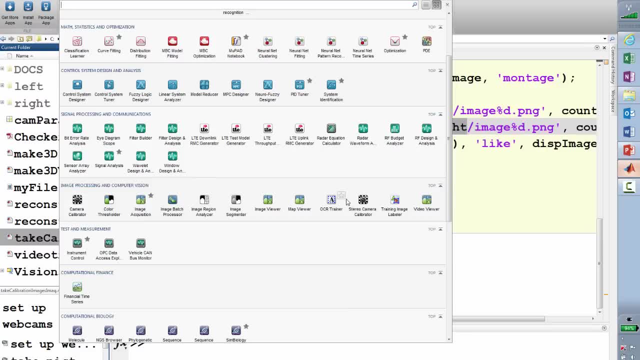 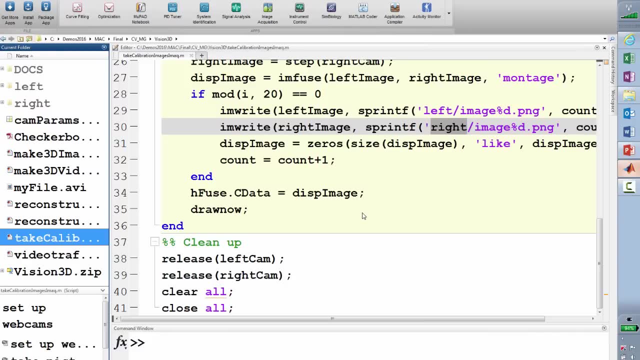 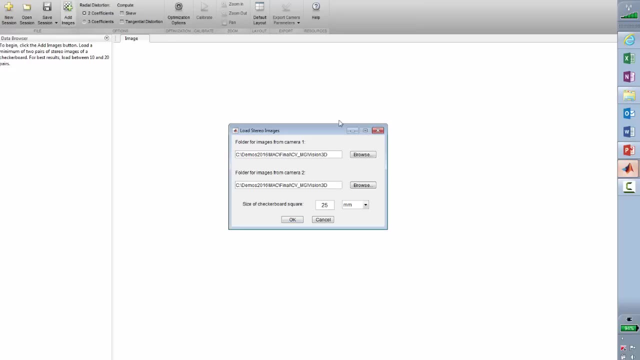 is for single camera calibration. We've got two cameras with us, so we'll be making use of the stereo camera calibration app, So let's fire that up And over here. the first step is to add those images, So I'm going to click on Add Images- Images from the right folder and Images from the left. 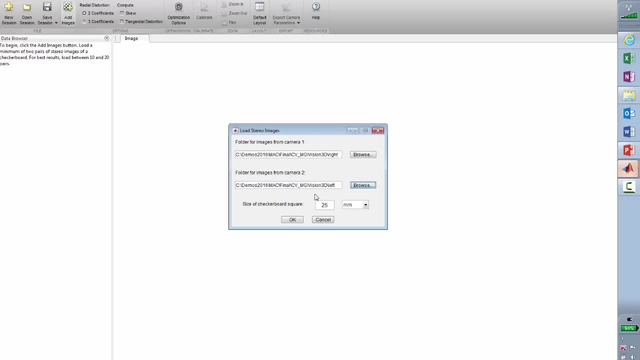 folder Select and the checkerboard size is about 33.5 millimeters. So you need to measure the checkerboard size and put those images inside that app. Okay, it is populating those images and these images will appear on the left-hand side over here. 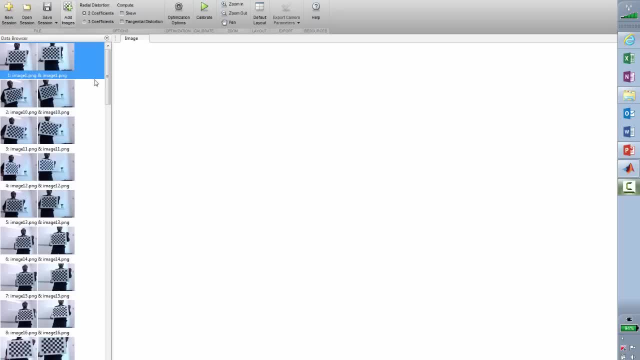 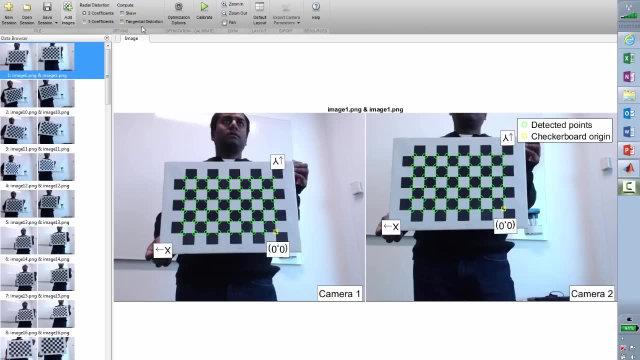 in the Data Browser pane. So once all these images are there, hit Calibrate. Now if you want to get rid of any tangential distortion, you make sure you need to check this box. But at the moment I'll just keep it simple and I'll hit Calibrate. So it's trying to calibrate both the cameras. 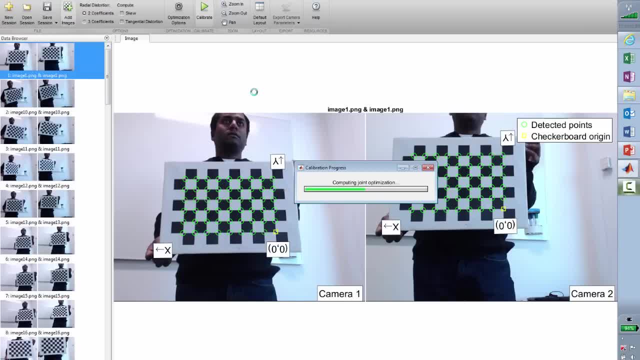 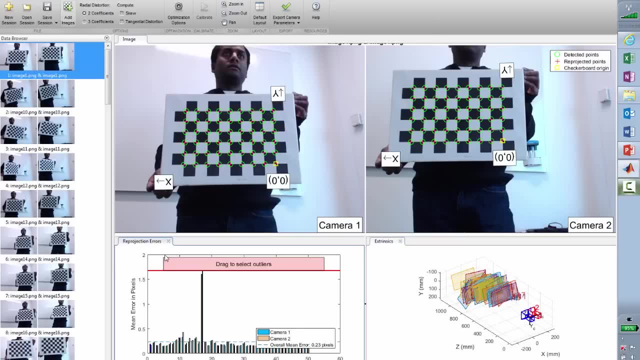 and in the meantime it will just give us some statistics. So it's giving some measurements, what's called the extrinsic and the errors. So extrinsic camera-centric or pattern-centric view how the cameras are seeing the pattern or vice versa and the reprojection. 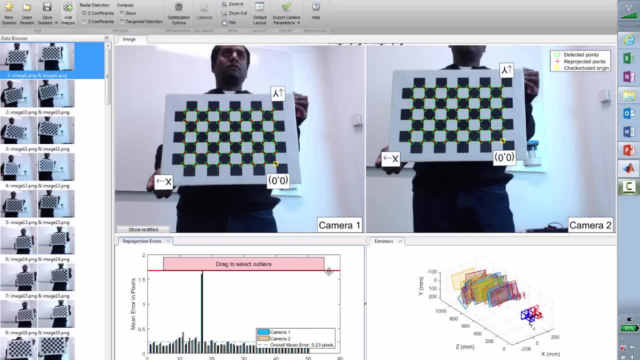 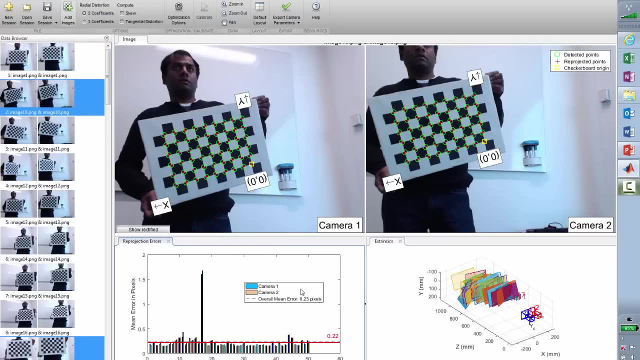 errors, whether it has properly found those checkerboard squares. You can play with those errors over here. You can play with the threshold and minimize. try to minimize those errors until they are appreciable to you. are they acceptable to you? So I'm just setting up that. 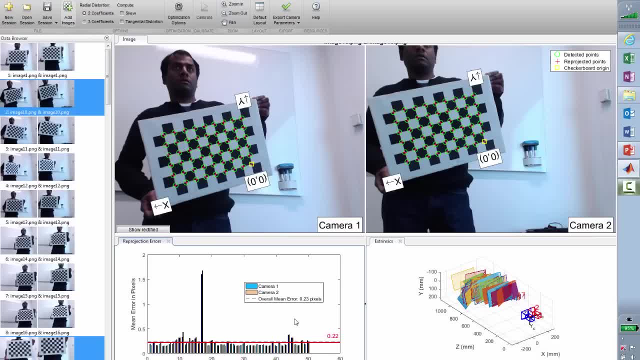 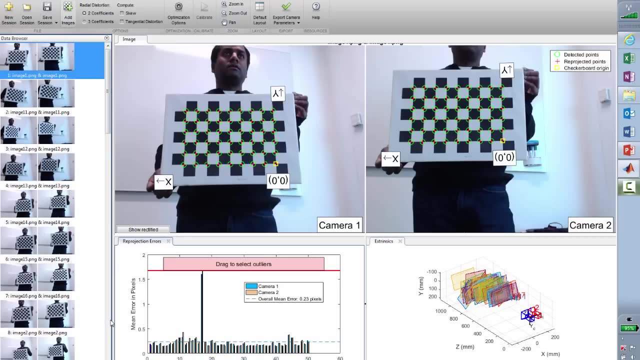 threshold value to somewhere about 0.22.. And once I move that threshold line, I'm just hitting Delete, So, which means that some of these images are selected over here at the left. So you want to remove them because they're having some high errors and you want to recalibrate the. 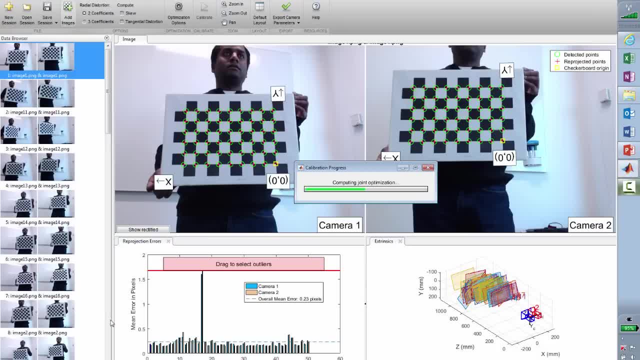 camera And that's the reason why that's the same purpose. That's the reason why I have taken 50 such images, so that you know my camera calibration pattern, or my camera is calibrated in a better way. You can move that even further If you want to just minimize even further. 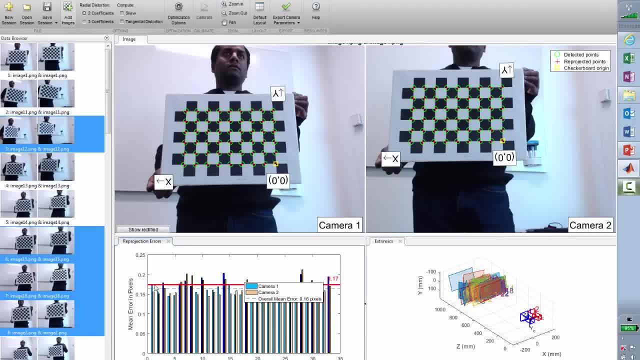 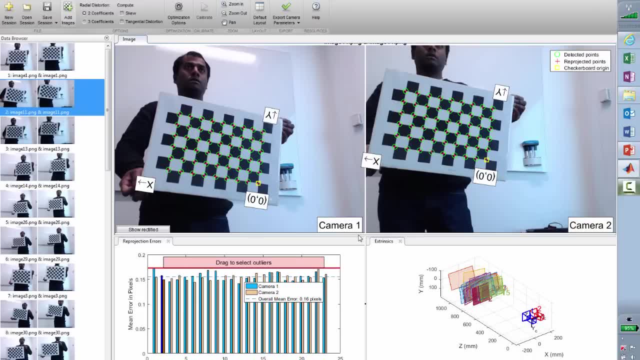 you can play with the threshold, see whatever threshold level is acceptable to you, hit, Delete and recalibrate the cameras. So it's up to you. Once you're done, once you're happy with the errors, error rates, you can export the camera. 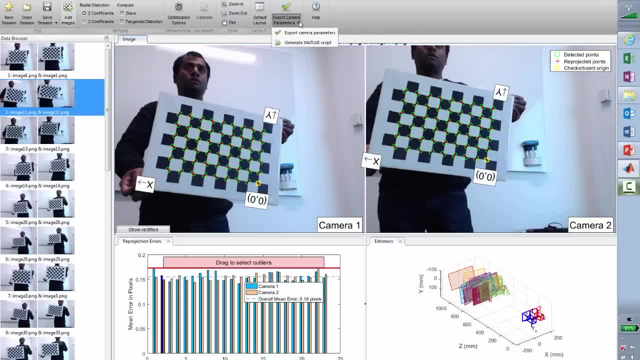 Now, in that particular green checkmark, you can export the camera parameters as a variable, or you can also generate the code. So for now, let's try to export those camera parameters as a variable. Okay, so once that's done, these variables will now be available. 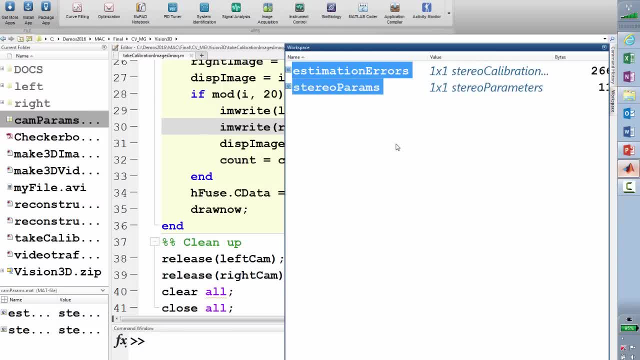 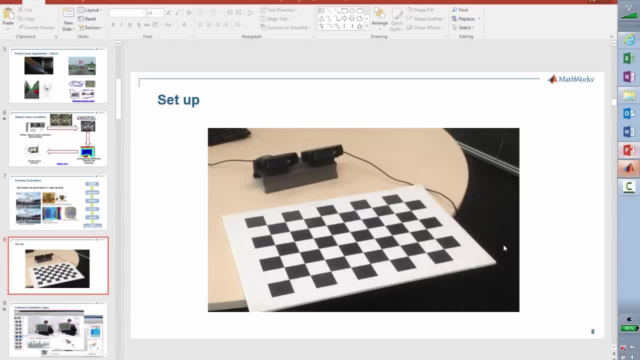 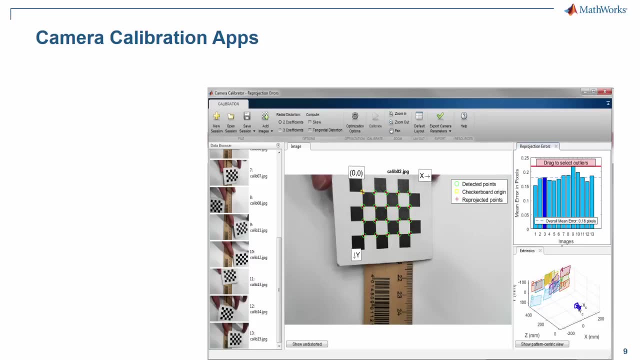 in the workspace. So these are the errors and the camera parameters- calibration parameters- which you want to use in the next step. All right, So let's try to summarize what we have just seen. There are different kinds of apps which are available If you're playing with single. 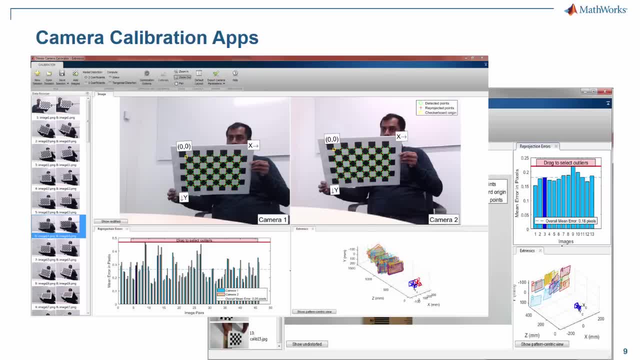 camera, you can play with the camera calibrator app Or, if you're having multiple views of the same scene, you can choose to work with the stereo camera calibrator app. Work with the threshold, find out an acceptable level of interest, error level of interest and then. 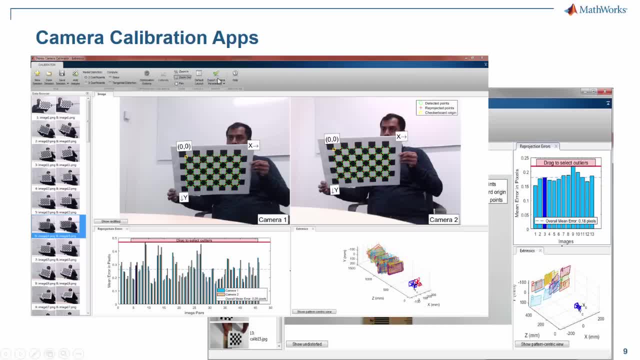 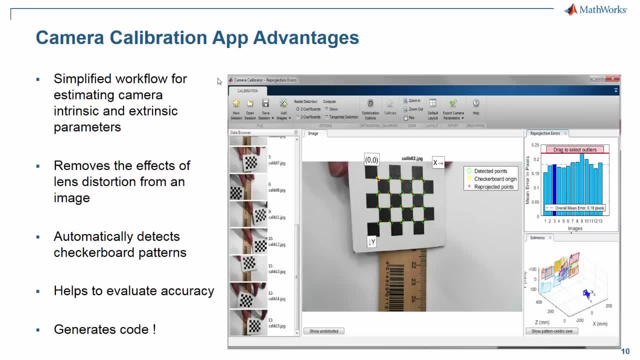 once you have acquired that, export the parameters onto the workspace. So the advantage of camera calibration app is a simplified workflow. It also removes the effects of lens distortion- tangential distortion. if you want to work with You can even select that particular checkbox. Automatically detects the checkerboard patterns, projects on them. 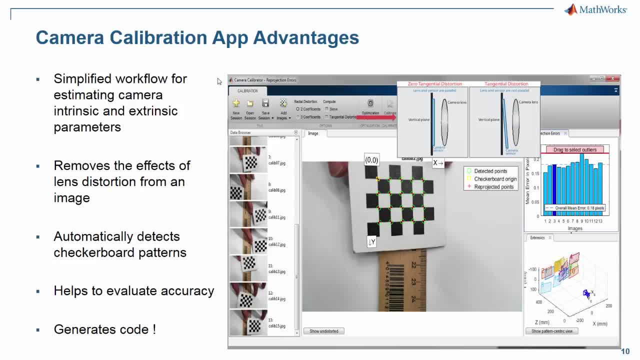 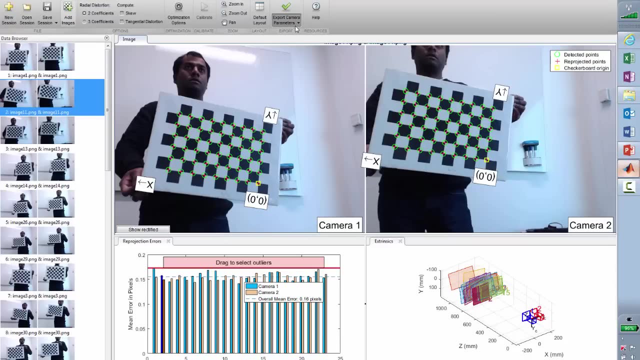 and also with the error levels, you can help improve the accuracy as well. But right now we have generated the variables which are available on the workspace. You can also generate the code. It is just the second option which is present over here. 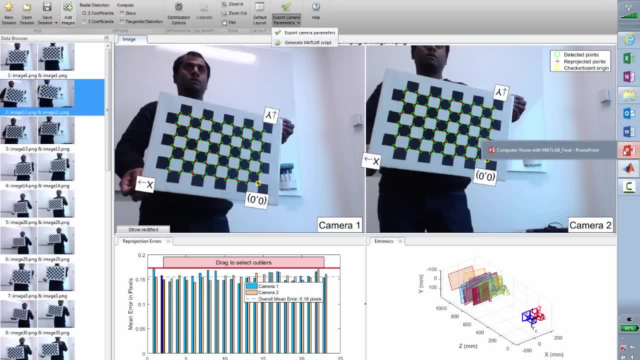 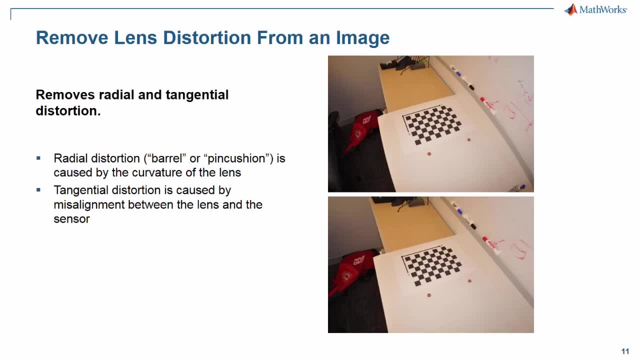 So you can also generate a MATLAB script. As for some more information, you can also remove the radial distortion and the tangential distortion, as in this example is seen. You could see in the upper picture that the table is a little bit curved In the lower. 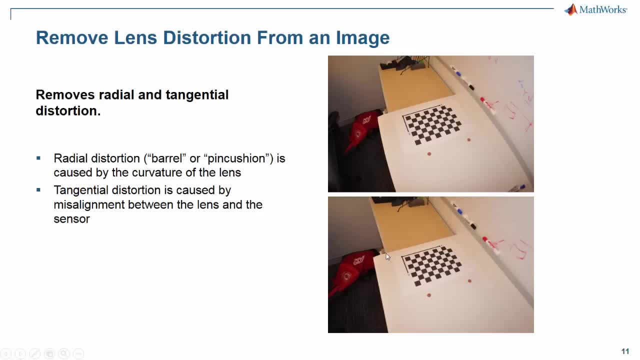 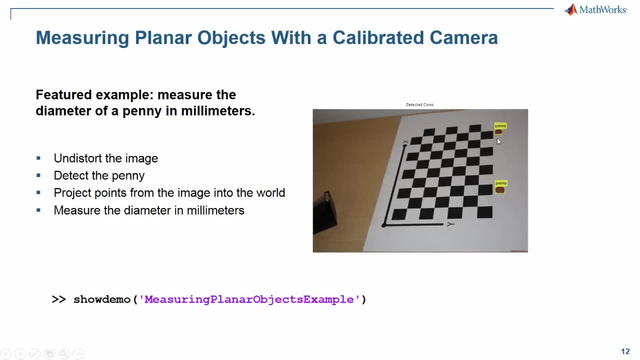 picture. after removing the distortion, the table appears straight. You can also measure the sizes of the objects. So in this case, if you want to identify what's the diameter of these two pennies, this is possible as well. Now, for those who are interested, I've introduced 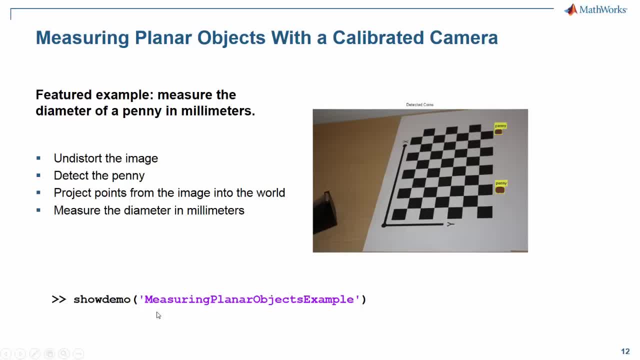 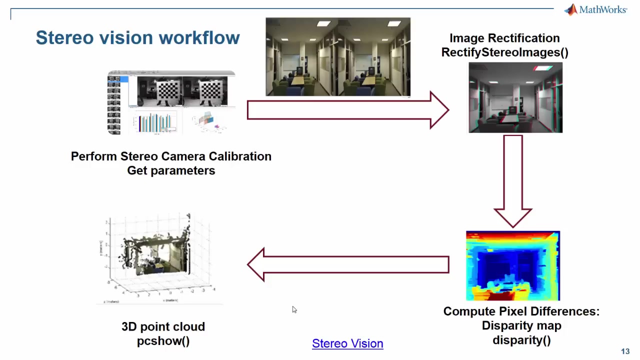 a shipping example comes with the product: measuring planar objects example. If you just type, if you just copy paste this particular show demo line onto your MATLAB command window, that particular example will open up and then you should see it in action. All right, so we are through with the first step and now we want to move towards the next step. 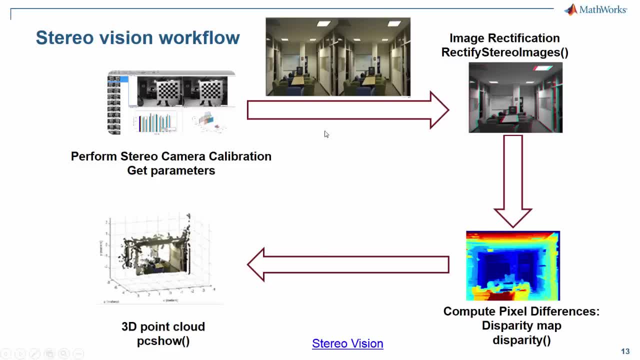 The next step is now. we want to start acquiring images live, and once these images are starting, once we are acquiring these images live, you're applying these parameters to do some image rectification: get rid of the distortion. and once the distortion is got rid of, you need to compute the pixel differences, how the two cameras are seeing an object with respect to. 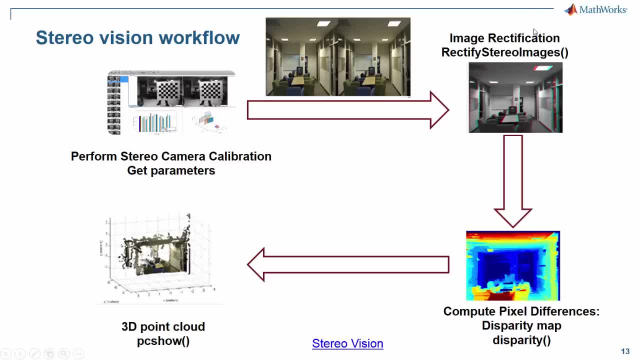 each other is any difference, and then put everything together to create this 3d point clap. So a couple of functions over here: rectify stereo images, disparity, map, pc show and so on. So let's have a look of how this could be done. 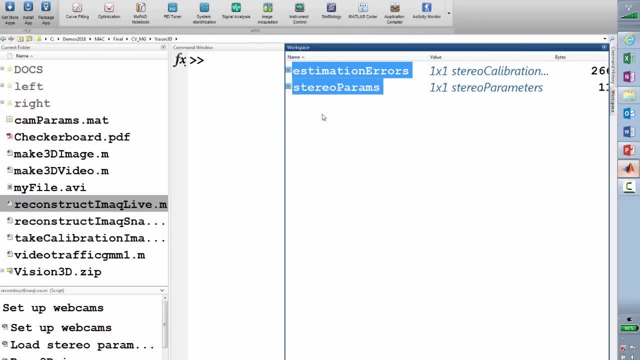 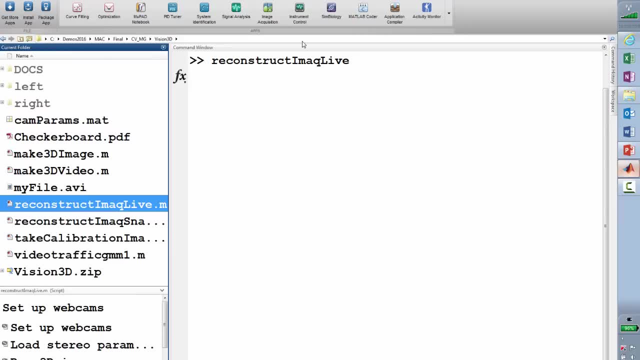 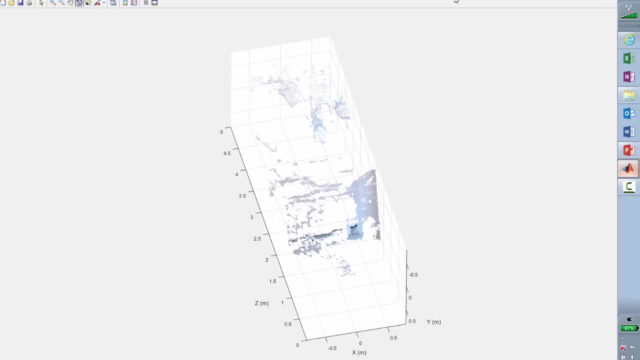 I already have the parameters in the workspace and I'm trying to apply them to a script. so I'm just running a script: reconstruct iMac life. Now, what this is going to do is going to get multiple views from the camera of the same scene and construct a 3d point clap. So I've got a 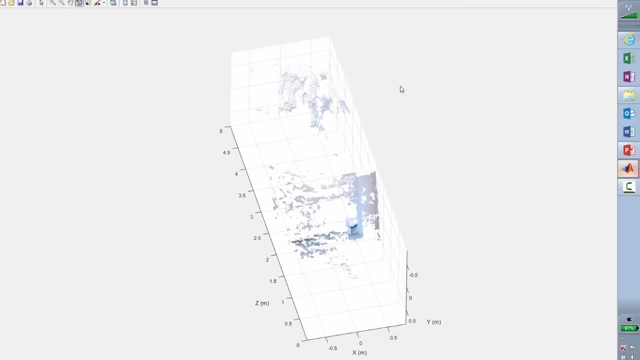 blackboard or a whiteboard beside me, and what you see over here, these are the pins So which have been, you know, stuck with a magnet on that whiteboard. I'm just moving in front of the camera now, So that's me, and you could see that it's able to also identify distance. so what you? 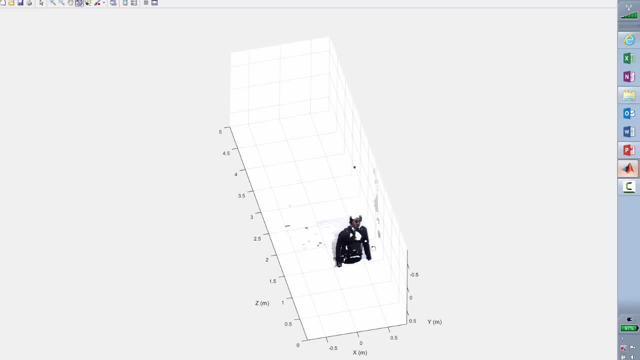 see on the z-axis. that is the distance in meters. I am just moving back and forth. maybe I just sit on this chair and you're able to see me there. So that's, it's a multiple views of that same scene, and MATLAB is able to construct a 3d picture of myself and the depth information is also there. So 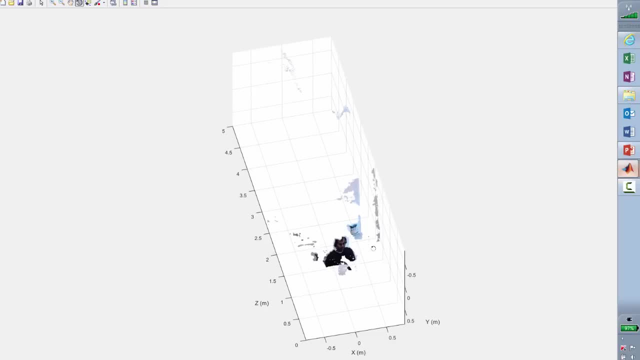 how far I am sitting from that camera. I can't go beyond that because there's a wall behind me. So that's what a restriction I have, but that's how Another thing is could be done to just moving out of the scene. I'm coming back to my seat. 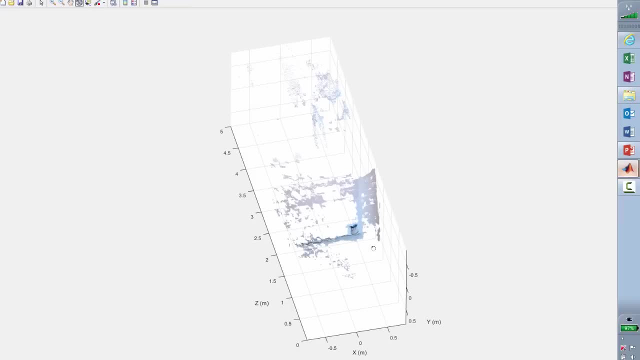 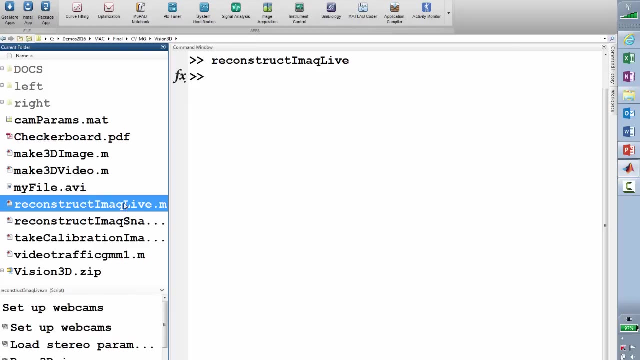 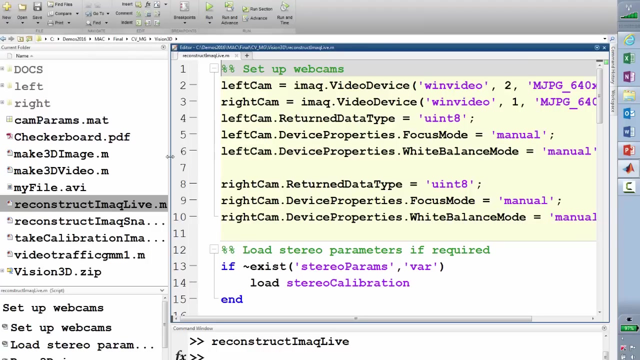 OK, Let's have a look of how this could be a Chief. let's have a look at the code. let's see how those functions which are introduced to you can be applied. I guess opening that script now. OK, that's the Reconstruction Scriptures. I'm pretty much you. 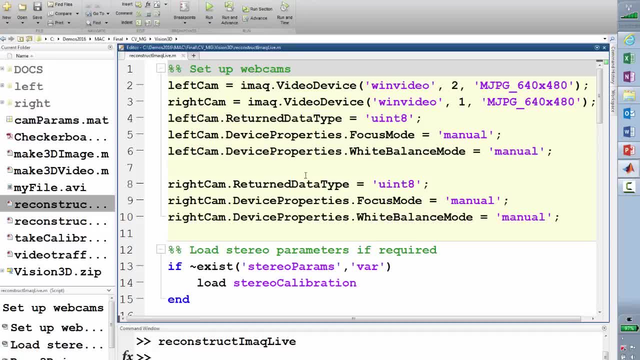 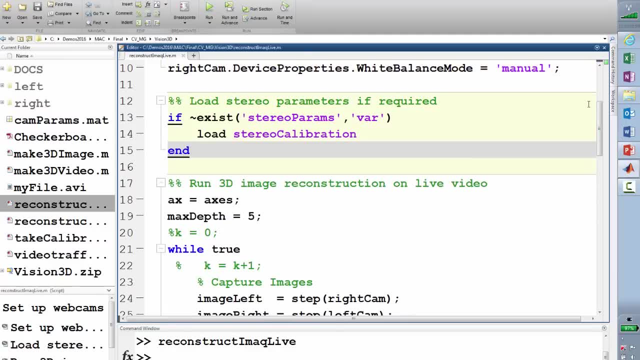 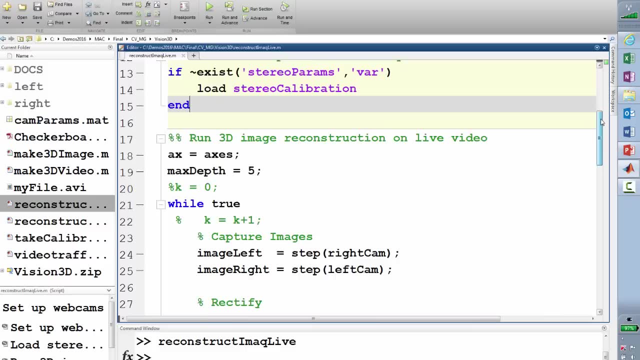 should be aware by now what the first section is doing: just setting up those two cameras and setting a few of its properties Over here. it's trying to see whether the variables are available in the workspace. If not, it's going to load them. I'm setting the depth to be five. 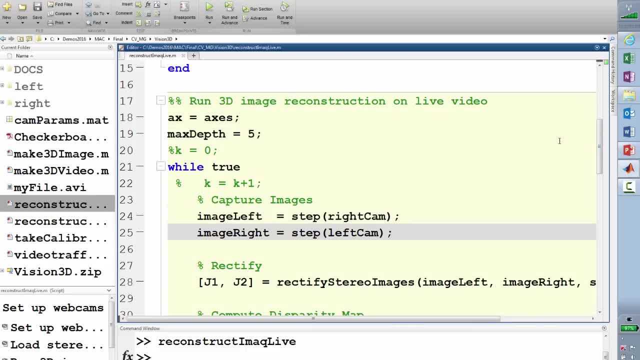 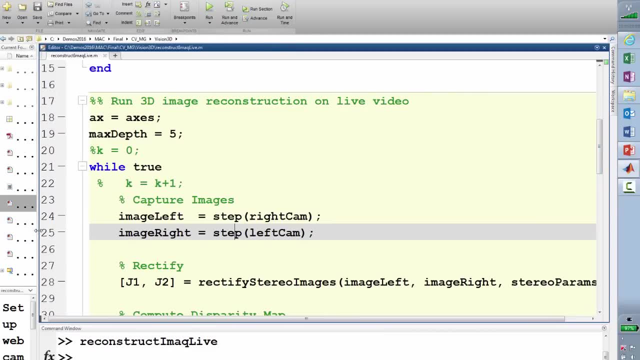 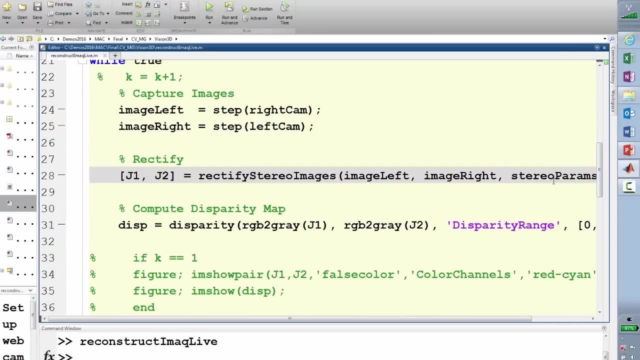 meters, This, applying these step functions to start the cameras acquire those images. I'm applying those stereo parameters which I got from the calibration app rectifying just one function to rectify those stereo images, one function to compute the disparity map. 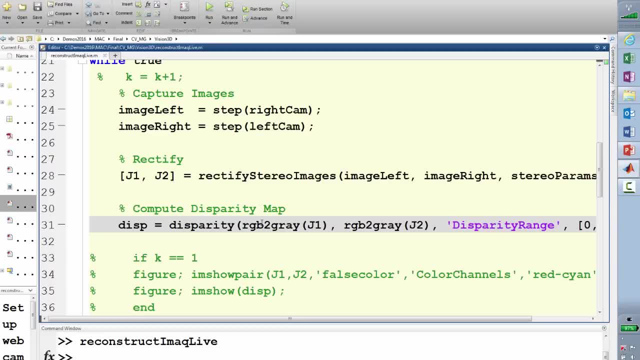 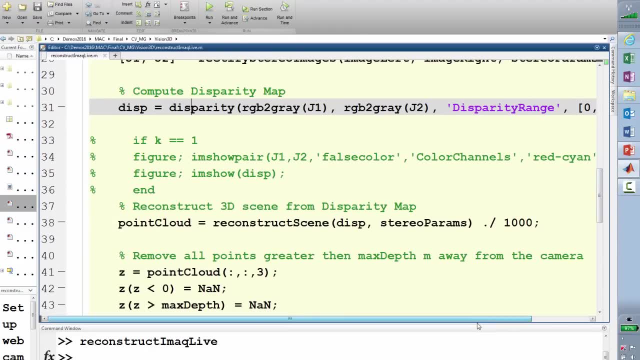 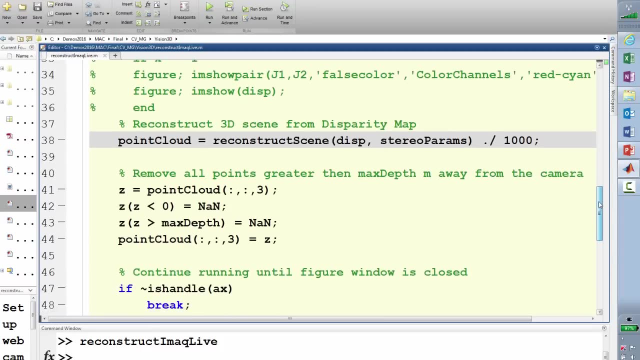 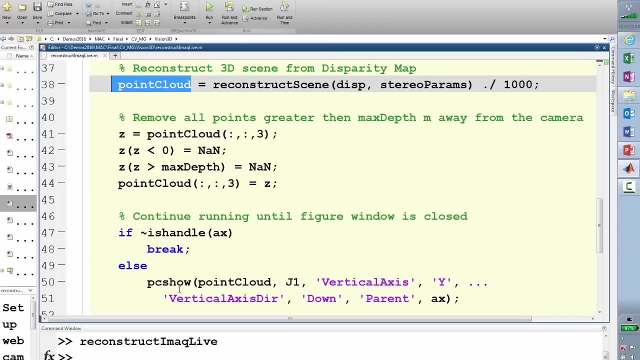 the output of rectify stereo images is the input to the disparity map And once that is parity map is done, you can reconstruct the scene using the reconstruct scene function, which you get the point cloud, And this particular variable goes into the PC show. 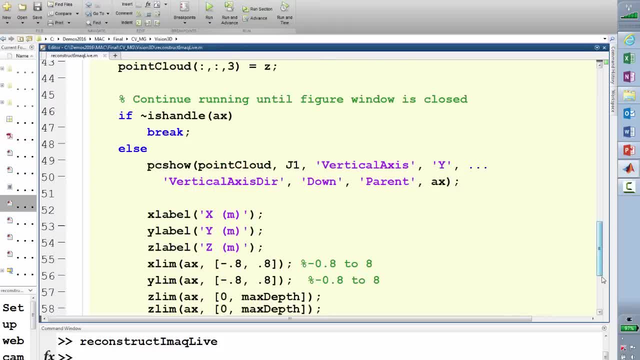 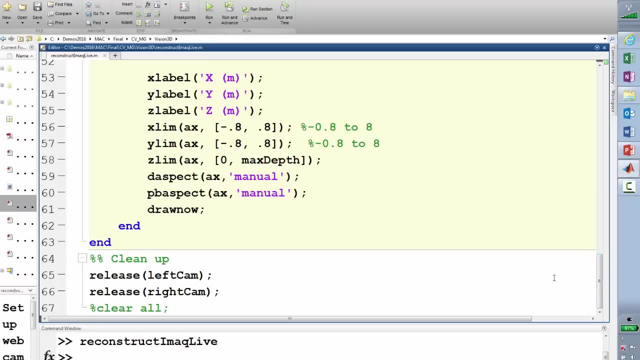 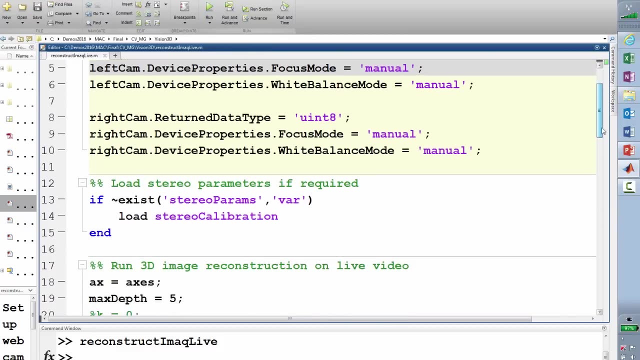 that you can display the point cloud. So all we did so, and what is coming up next is just visualization. So I'm just adjusting the visualization, setting the limits and so on and so forth. So just simple steps. The first section: you need to set up the cameras, fire the cameras. 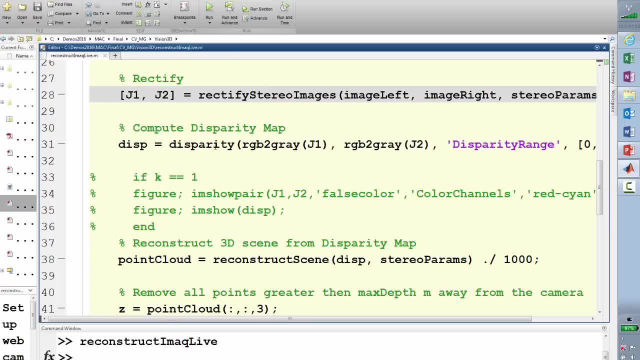 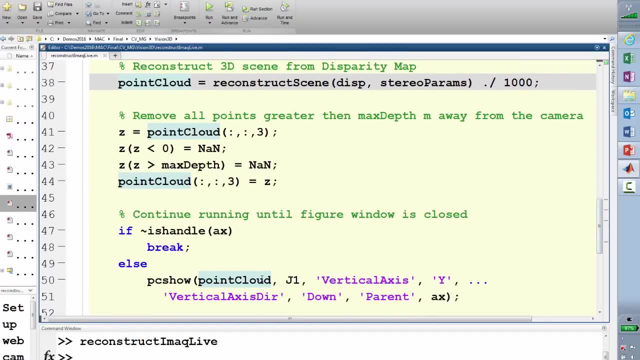 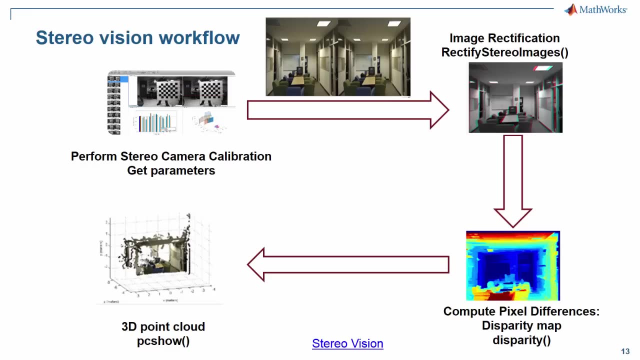 and that's how three functions rectify- see your images- disparity map. All right, Four, reconsider the scene to get the point cloud and PC show to display the point cloud. Okay, So that's what we do. That's what we did. That's how. those are the four steps. 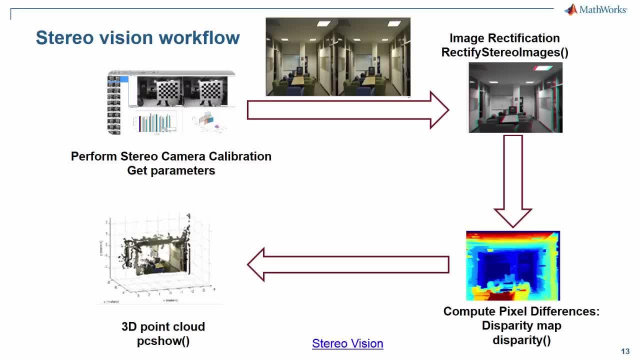 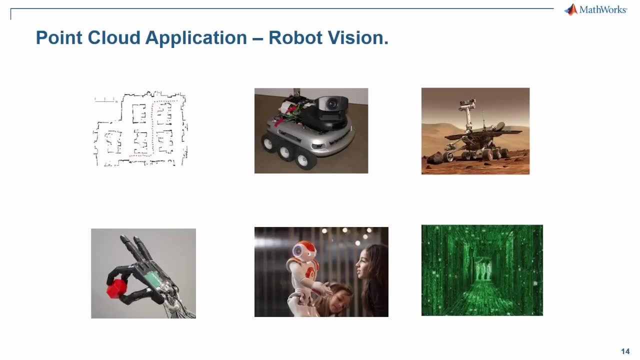 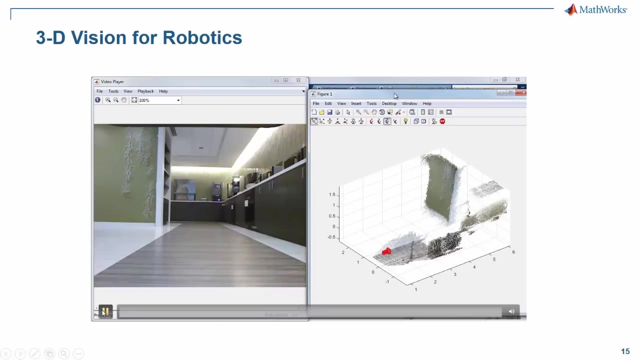 And the associated functions, how you can tie them together to construct the 3d object from multiple views of 2d scene And point clouds can also be applied to robot vision, So one such example is this particular video. so there was what we did. this was done on in our 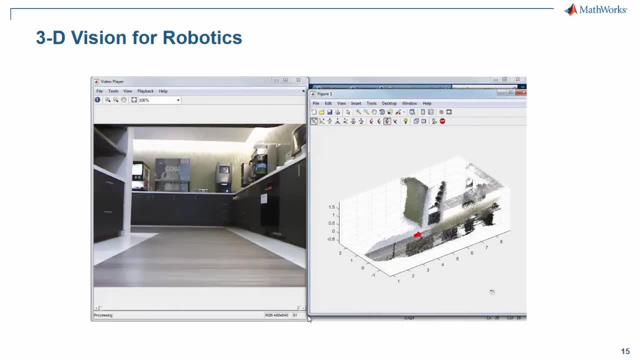 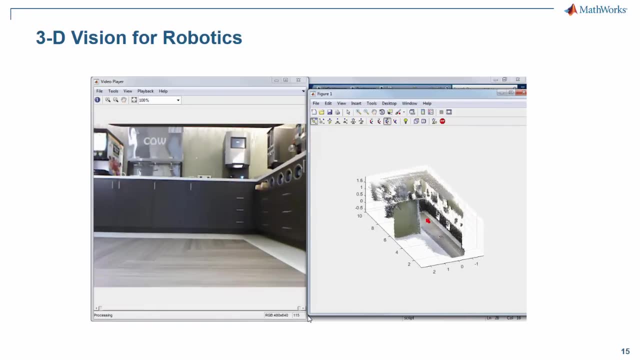 math works kitchen. Um, a robot is traveling with with a camera fixed on its head and as it's traveling it's trying to reconstruct the scene on its right. so you can see that, if it's, if there is any danger of collisions, also sensing that, 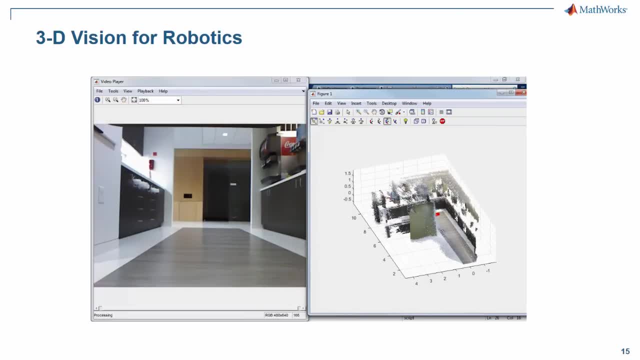 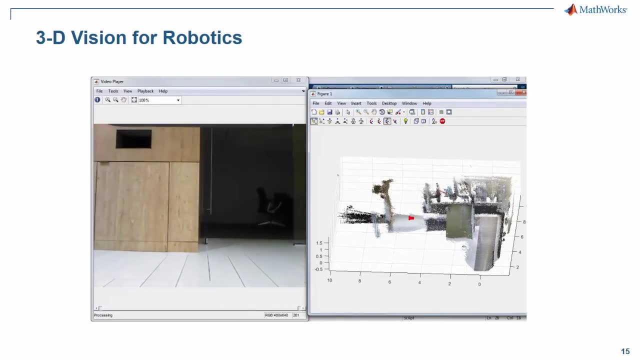 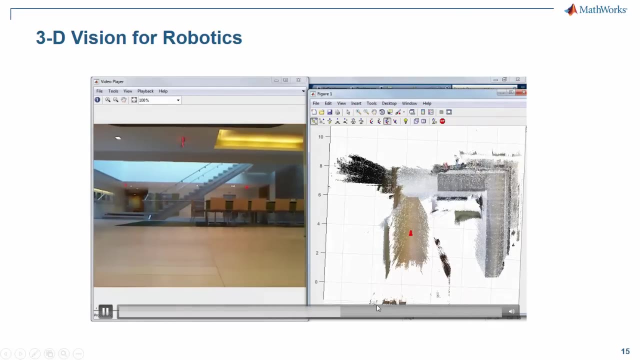 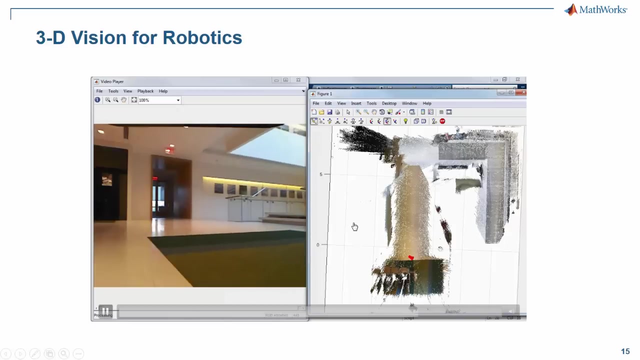 it's able to change the path. it's coming towards the doors. as it goes near there, it's able to change the part. now you see over here how the scene hat is getting reconstructed. similarly, as it goes near the chair, it's able to change the path. so, as it, as it's moving through that region, the scene is also. 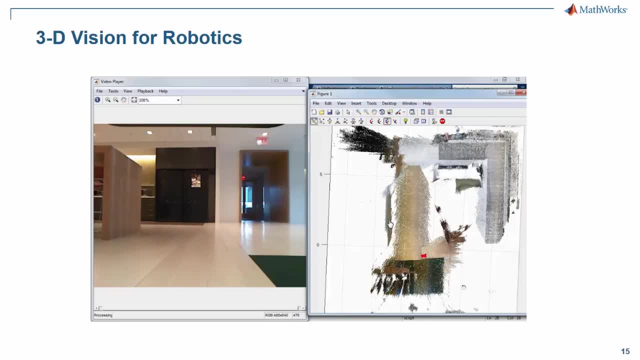 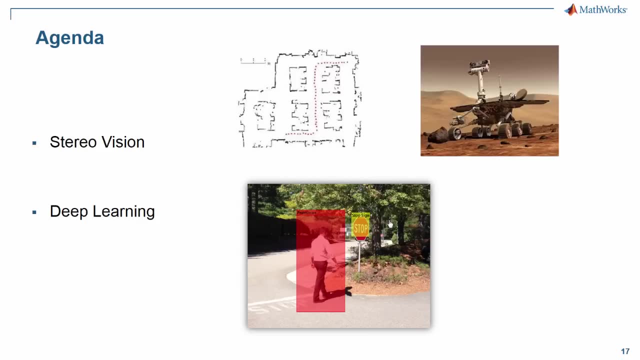 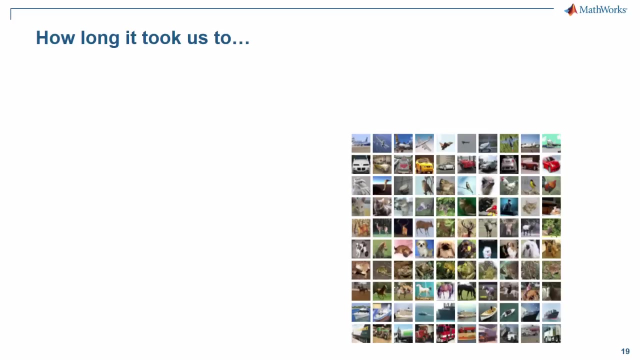 getting reconstructed. so this is one of one of the examples how 3d vision can be applied for point for adas systems as well. okay, so, having seen stereo vision, let's go to the next part of our talk, and that's about deep learning. now, before just we jump into the deep learning concepts, let's try to play a game, and in this, 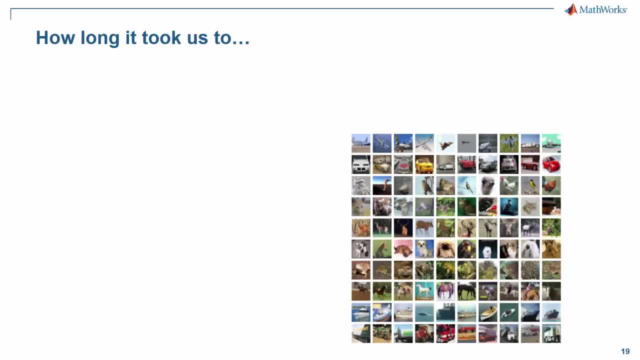 game. there is only one rule: you have to be honest, okay. so the question is: at what age does a person start to recognize the difference between a car or a plane? maybe some of you must have guessed. maybe two years, three years? car or suv takes a while. eight to ten years, maybe. 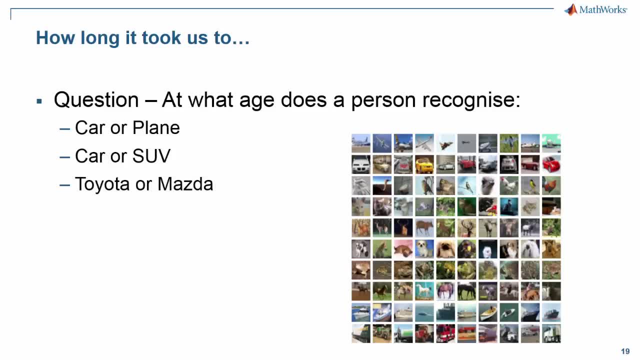 toyota or a master, it takes even longer. so a human being, it takes he, a human being, takes longer to recognize. it takes so long to recognize the differences between the two objects. it takes so long to recognize the differences between the two objects. so if you were to come up with some kind of a surveillance system, say for example, we've got. 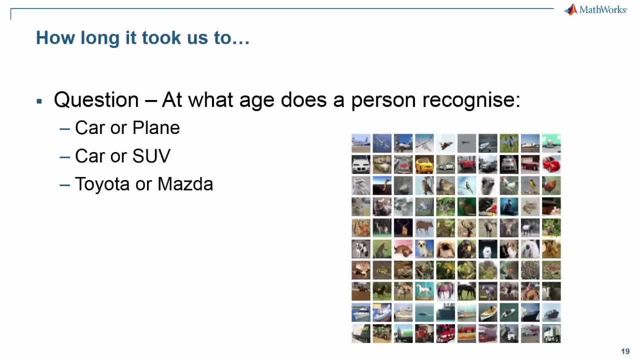 parking bays for cars and suvs. this if you want to just come up with this surveillance system with human not in the loop. you want to just build a machine. you can't just wait as long as a human- say 10 years- to recognize the difference between car or suv, to make sure that appropriate bays are. 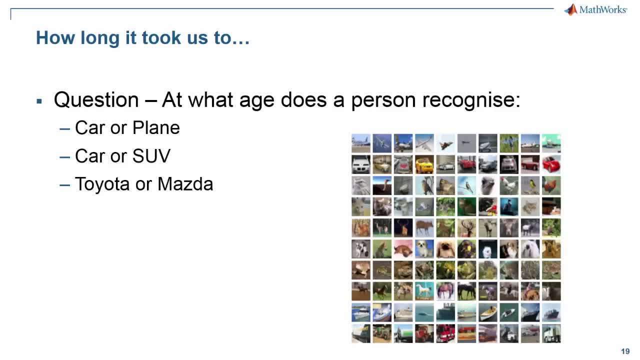 full. no, you can't just wait as long as a human- say 10 years- to recognize the difference between car or suv, to make sure that appropriate bays are full. no, you have. you want to get something quicker, and to get something quicker. that machine needs to learn, learn faster. 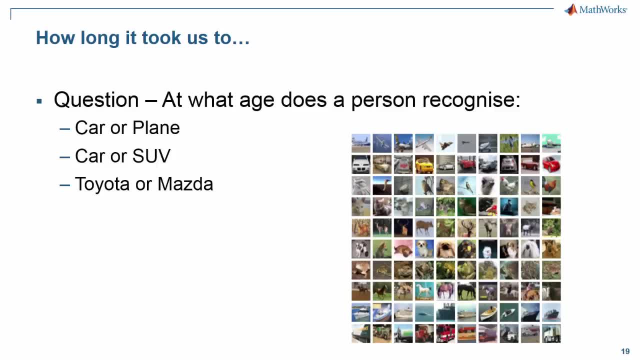 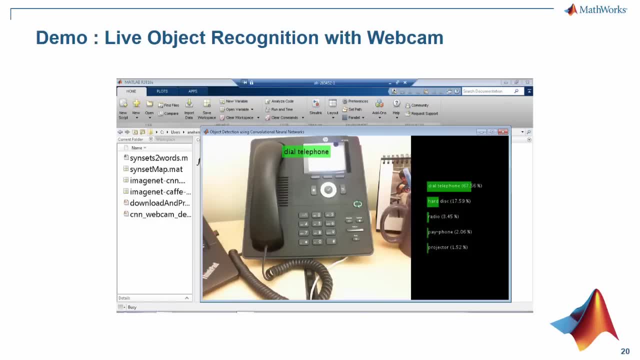 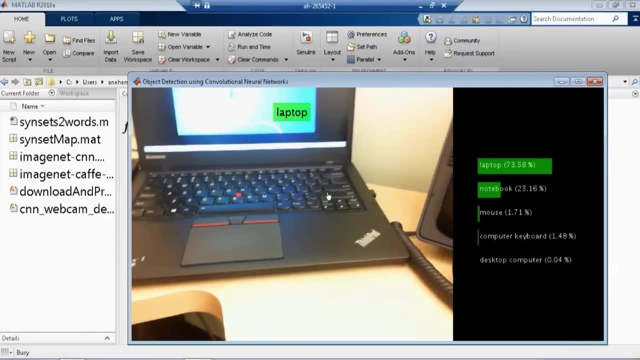 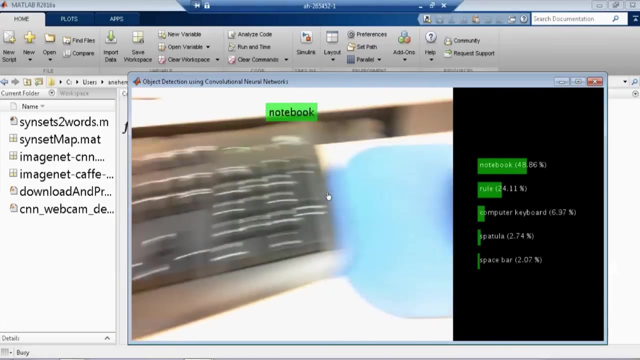 learn all types of cars, identify all types of cars, identify all types of suvs, so on and so forth. so, with this in mind, here's something which we have built to identify the objects. it's a deep learning system. it has taken into account different types of objects, namely computer. 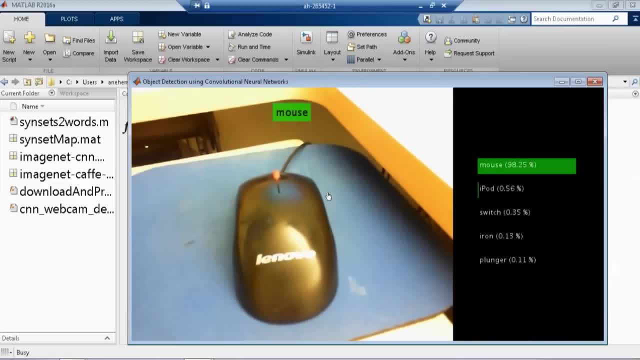 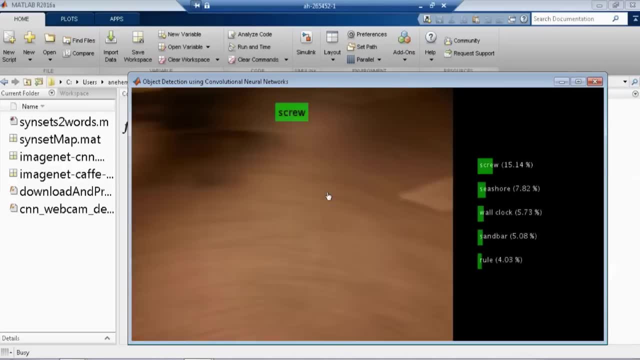 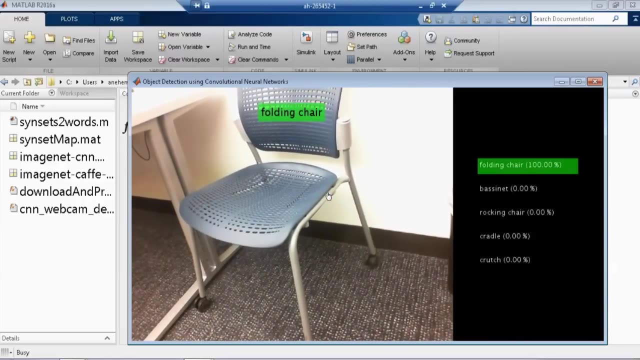 keyboards, uh, ipods, ipads, mouse and so on- and, with this in mind, when it's trying to, it's presented with a live webcam. when the video is getting acquired live, it is doing some detection and most of times, as you have seen, this detection is correct. alternatively, this is another one where 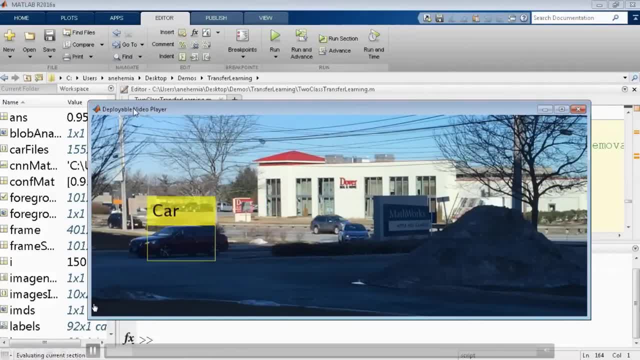 alternatively, this is another one where a live surveillance system is beingная incident and, if is being built, what type of vehicle is entering in MathWorks premises? maybe a car or an SUV, and so on and so forth. So what happens? in this case, it feels like. 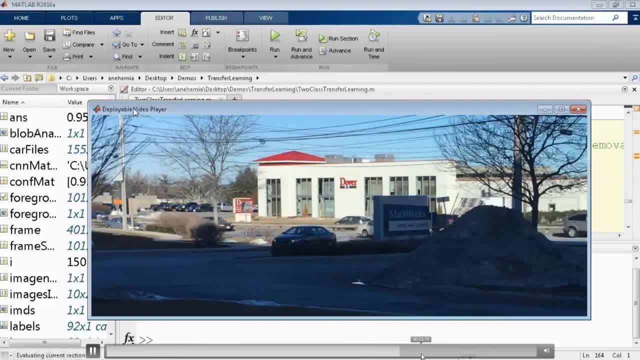 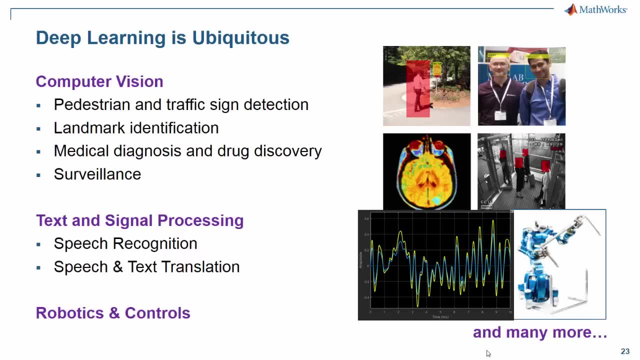 okay, it has identified that as an SUV, and so on. So object: detection, surveillance, deep learning is everywhere. It's for computer vision, for pedestrian and traffic sign detection, medical diagnosis, surveillance, landmark identification, fraud detection, for speech recognition and text recognition, even robotics and 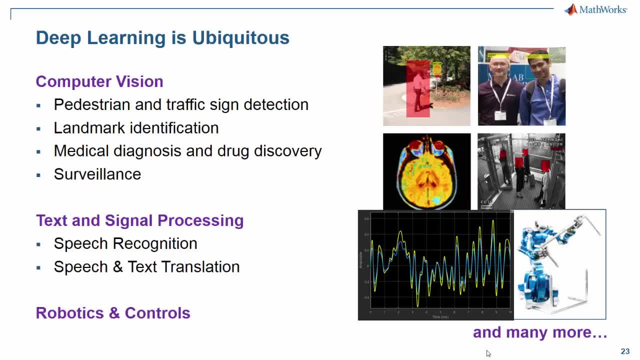 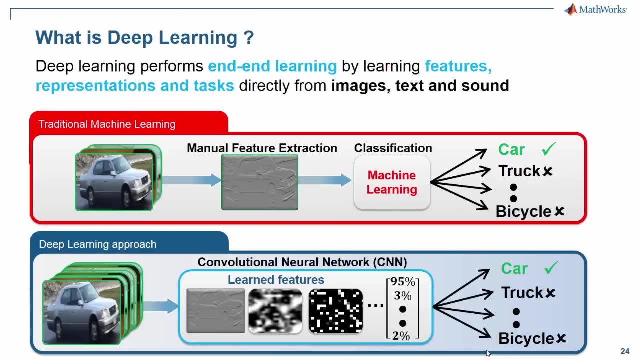 controls. So there are many areas where deep learning can be applicable, can be useful. So while we are on this deep learning topic, let's try to answer a few WH questions. What is deep learning? Why deep learning? How to do deep learning? We have seen machine learning. 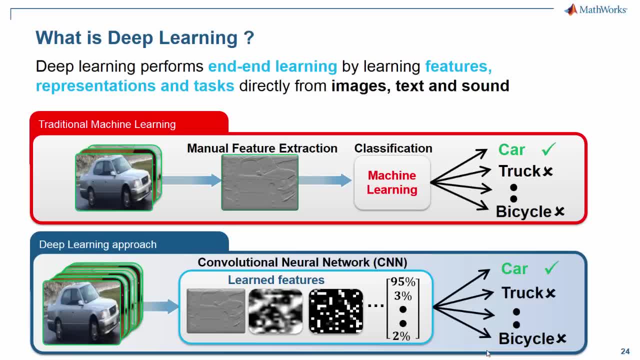 techniques or data analytics and machine learning seminar a few seminars ago, and what we have seen over there is for machine learning, if you're playing with images. what we did is we extract these features and we push these features through that classification learner app, which then builds a network for classification purposes. Now why doing? 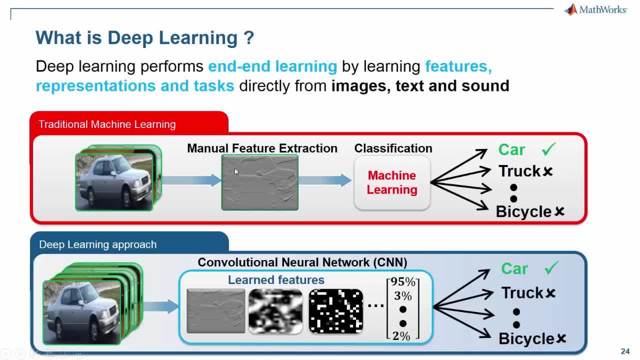 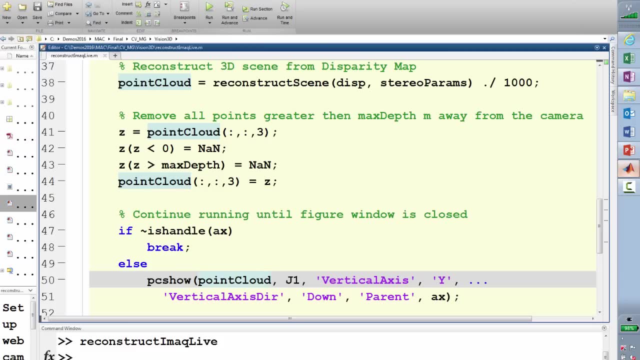 these are feature extraction. this is all manual, manual in the sense we need to understand, we need to select which particular feature extraction algorithm is required. And it's not that we don't have these feature recognition extraction algorithms. These are present and most of these algorithms for feature. 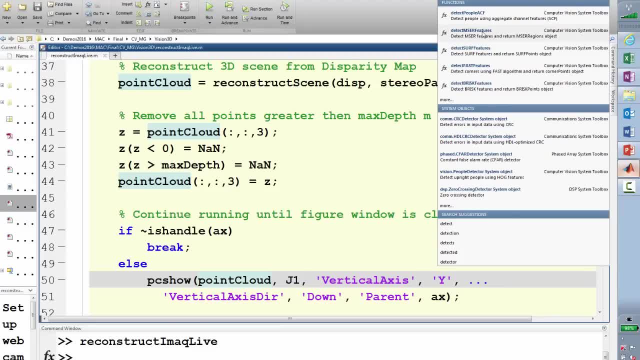 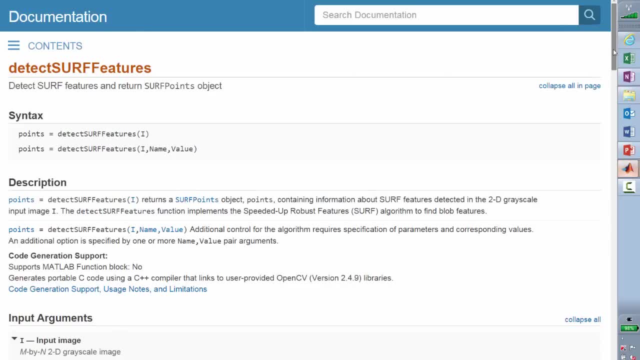 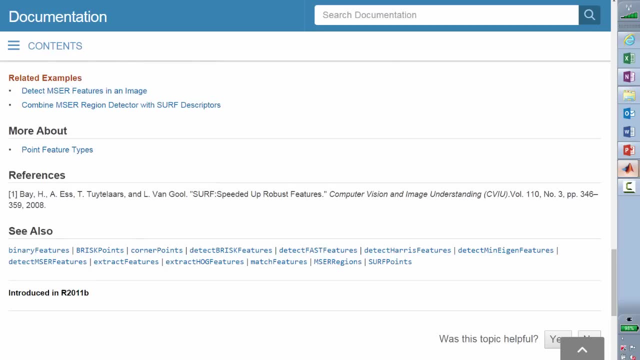 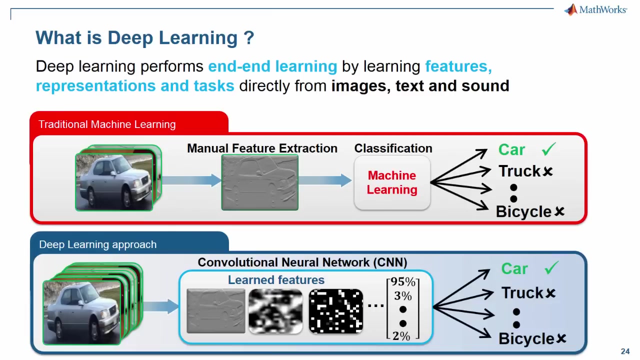 extraction or feature detection. They start with the world, detects, it detects or detects MACR and all those things. They're all a part of computer vision system toolbox. So these particular functionalities are available Now. so you have to manually go through the process, acquire an image, extract the features, identify a classification term and then push to. 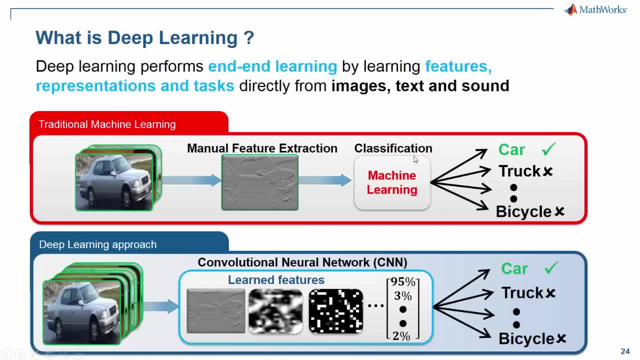 the classification on an app so that a machine is being built. However deep learning is, some is called as end-to-end learning. You're giving it a bunch of images and that particular deep learning approach is like: it comes up with its own filters, acquires, comes up with its own. 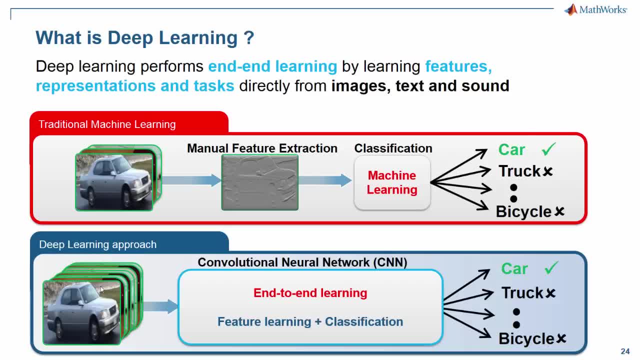 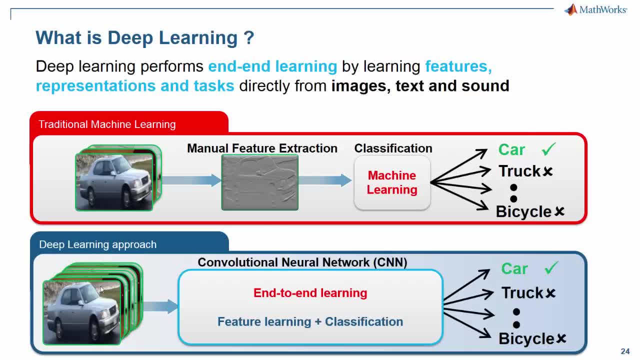 deep learning network, which is popularly called as a convolutional neural network. Once these features are extracted, they are then presented to the classification stage and further which the classifier is built. So this manual approach is not there in it's in a deep learning, The 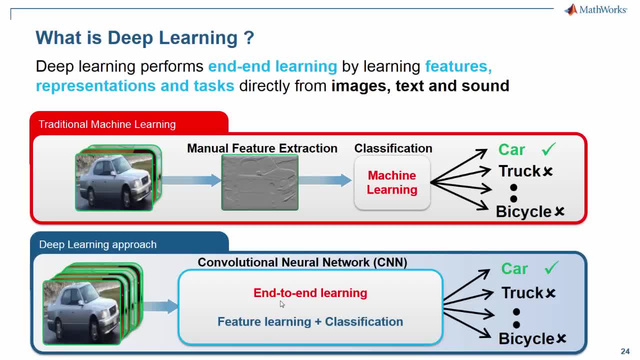 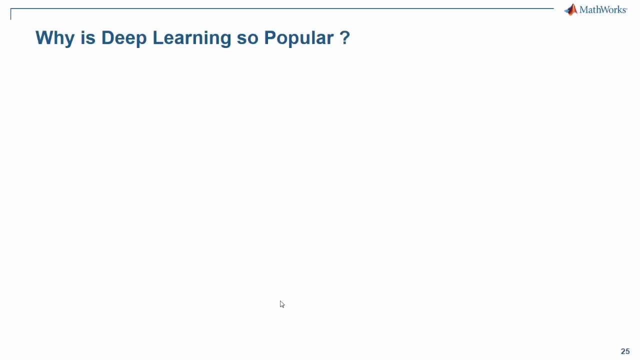 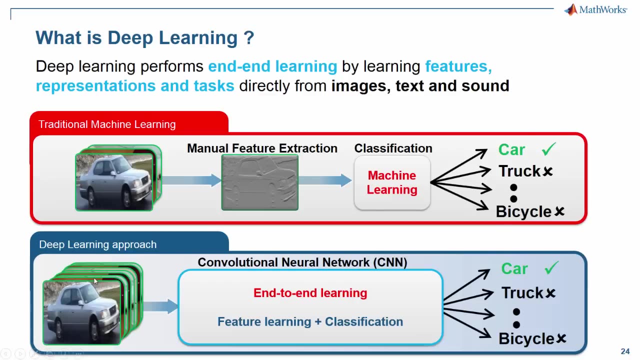 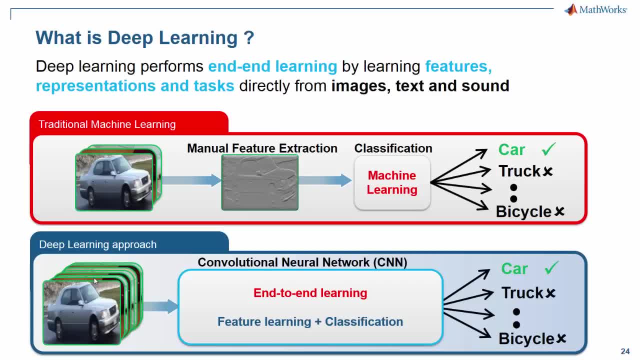 surveillance or for uh identification purposes- car or SUV identification purposes- you need to take into account all the different models of cars, all the different models of SUVs And if you want to go do some identify some other vehicles, you need to take those different models of the vehicles. 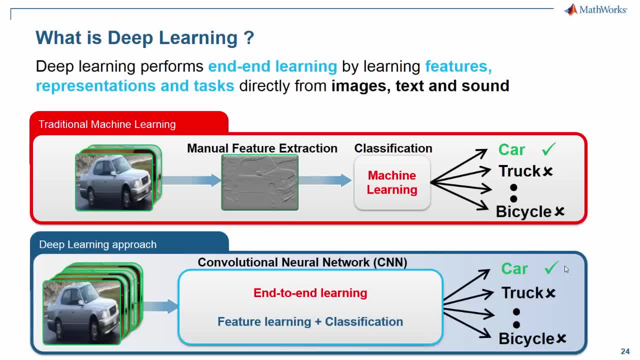 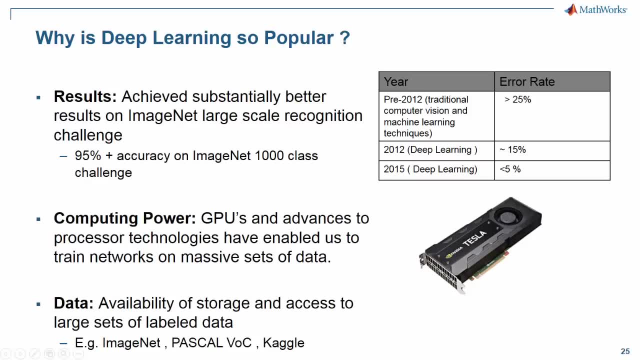 as well in, in which means you have to work with number of images. so for this, you need to play with large amounts of data. and if you want to play with large amounts of data, where can you have that data? where is this data present in today's world? 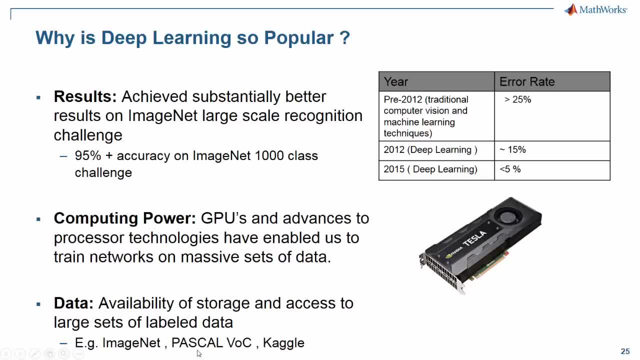 there are lots of data storage facilities which you can connect to. you can connect to a lot many databases and you can download such labeled data which you can use for training your deep learning network. Now, while you're playing with lots and lots of data, I mean there are also resources which you can use for. 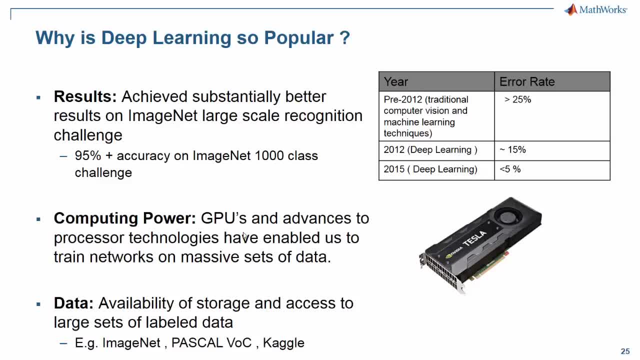 training computing power. we've got a lot of. we have a lot of these fancy computers with multi-core, multi processor technologies or even GPU cards. we have access to clusters. there you can use these facilities, you can use these resources to build this deep learning model. and because of all these things, because the availability of data, because 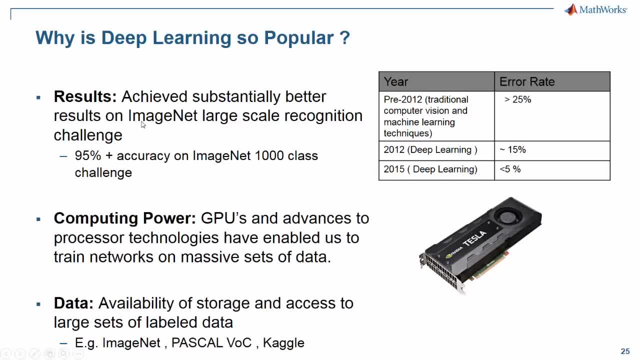 of computing power available to us. the results which are being achieved now are substantially better and, as you can see, there's some estimates which are placed over here. pre 2012, the error rate was greater than 25%, and that has substantially come down over the last few years. 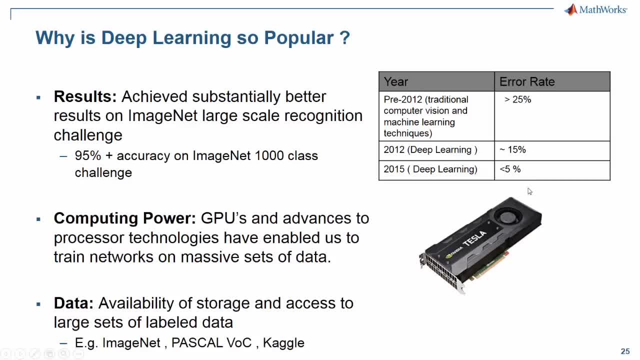 2015 it was less than five percent and is getting better and better. so, because of all these resources, because of all this data, all these data sets which are there, it is very easy to get the data sets, it is very easy to work with such data sets and it is now becoming more and more accomplishable that you can get. 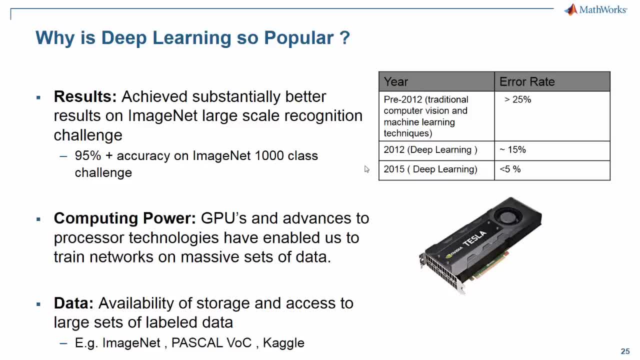 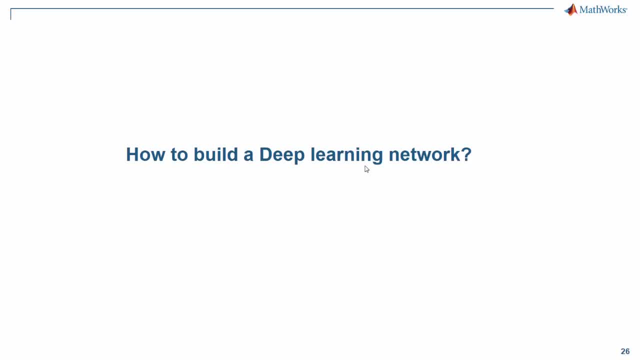 you're getting better results. So deep learning is gaining is becoming popular. it's learning can also be seen as an evolution of machine learning. so how to build a deep learning network can matlab does? matlab has these functionalities to build these deep learning network. so in the surveillance video which you just saw, which you just saw, which was identifying 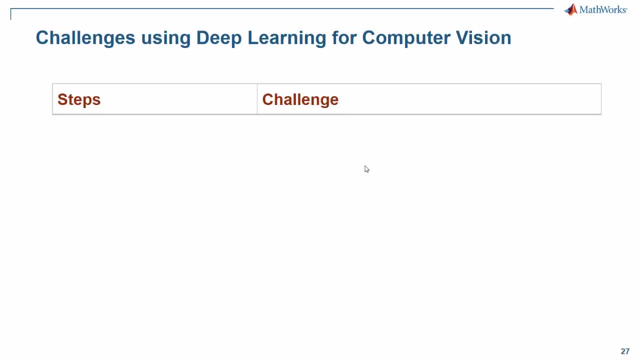 whether it's a car or suv, the different steps which were taken into account. if you're given a video, the first step was working on each frame. so from the video, apply an algorithm to extract the frame. the frame may be clear, may not be clear. you might want to do some pre-processing. 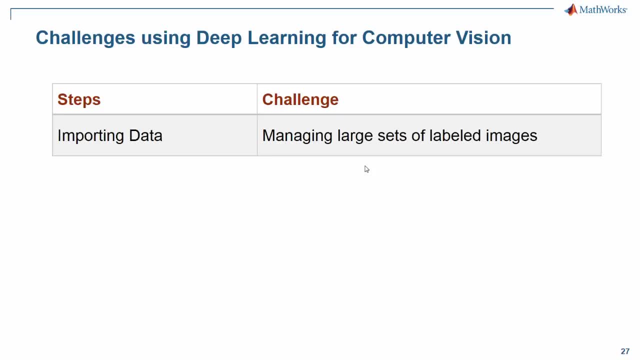 on the frame, something like you might want to do resizing, contrast enhancements and so on and so forth. so once you have that data, you want to extract frames, you want to do some pre-processing, say a resizing or data augmentation. once you're through with this pre-processing, you need to push those images- labeled images or frames- through a network. you 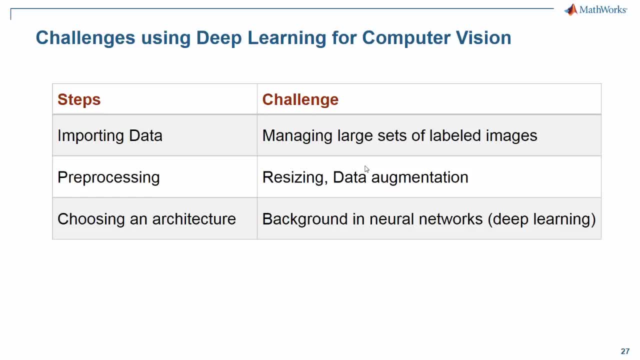 need to. you need to know a background in the neural networks or the deep learning and once you have you have, you have built your architecture for the deep learning network- you need to push that data through that network for training and classification. now, because you're playing with large data sets, you may want to require, you may you're compelled to use some. 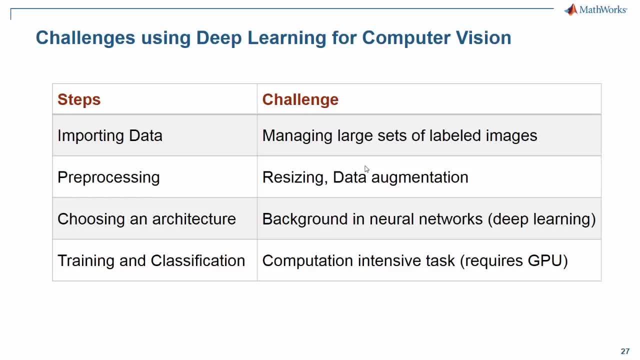 some resource which can do the computationally, which can do these tasks which are computationally expensive, something like the gpu or a high power machine, and you need to repeat these processes again and again. so you need that needs to be iterated. so, whatever you build, whatever you, 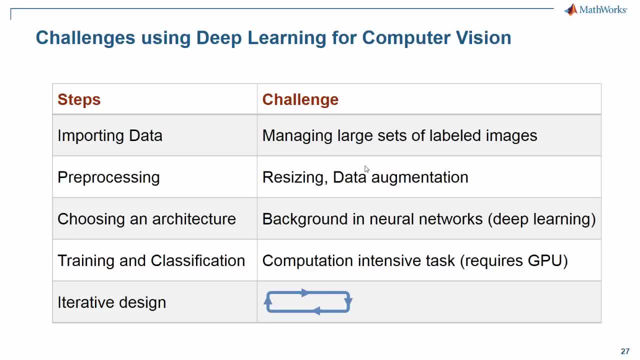 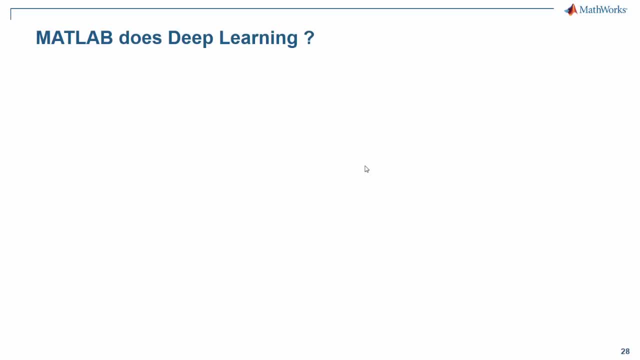 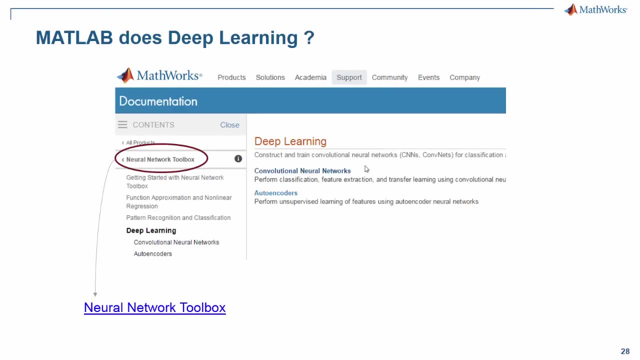 work with. it has to be iterative. so there are different challenges in deep learning for computer vision. so let's see how we can overcome these challenges. so does matlab do deep learning? yes, it does, and the deep learning functionalities are now a part of the neural network toolbox, inside the neural network toolbox. 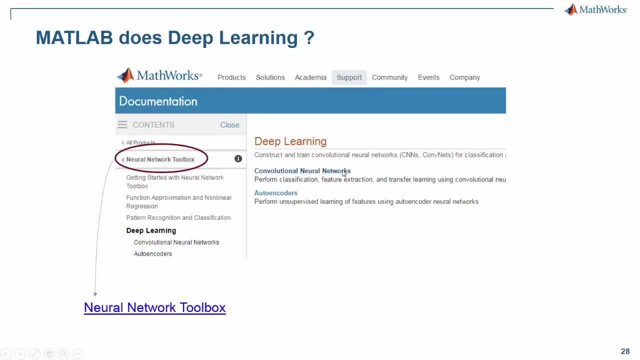 you can search for deep learning and you're given two matches: how to build or how to build the convolutional neural network for your own architecture, and also you can work with encoders. okay, so that's just a brief. uh, that's a brief theoretical slide of what, uh, convolutional 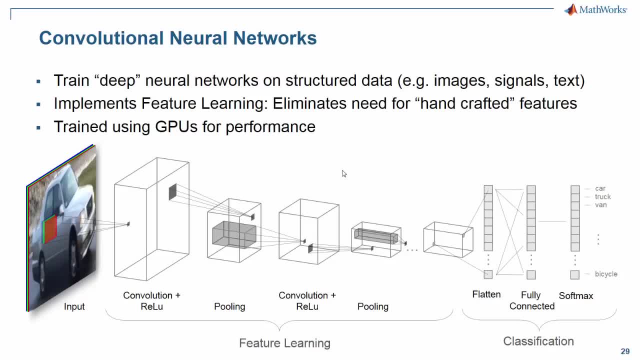 neural networks, mean or cnn. you've given an image, you have a bunch of images you. it comprises a convolutional network, typically comprises of two stages. the first stage is a feature learning stage and the second stage is the classification stage. in the feature learning stage, the network needs to come up with different types of opportunities for Ai models in the 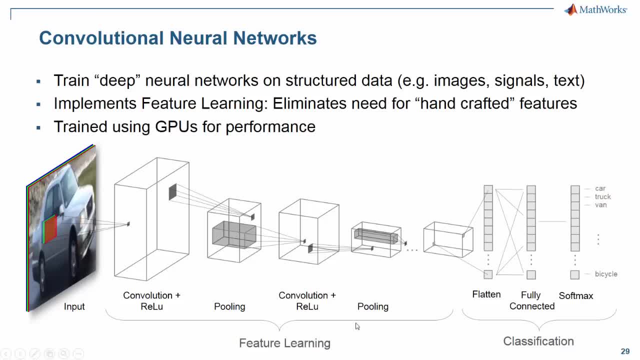 society. it takes months to sore out all the ruim nutrition, all these bases here, to pull these builds upmaa. look, you've got it a minute and i don't recall that's what this one is saying. we need to 확인 of filters which do the convolution operation and that's the reason why it's called as a convolutional. 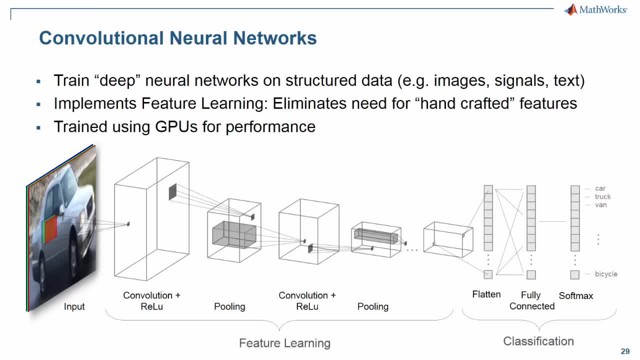 neural network in this convolution of their multiple filters which have been taken into consideration, and all these filters come up with different features. they extract different features from these images and typically in the feature learning stage it has got different sub stages. in a theoretical sense it's some. it could be convolution stage, a relative stage, pooling stage. 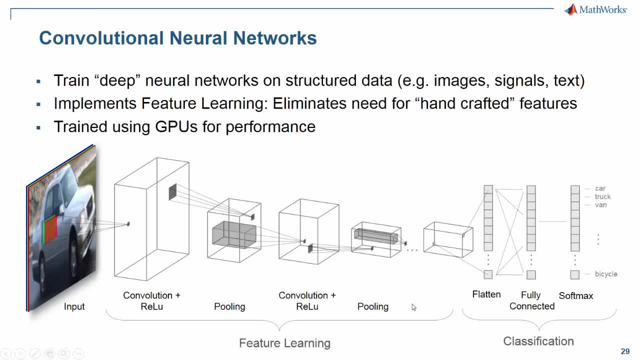 and so on and so forth. so at this, uh, in this particular slide there, i have just shown two such sub stages, but there could be many, many more. and once the network is through with this feature learning stage, it goes, it goes to the next stage, that is, a classification stage in the 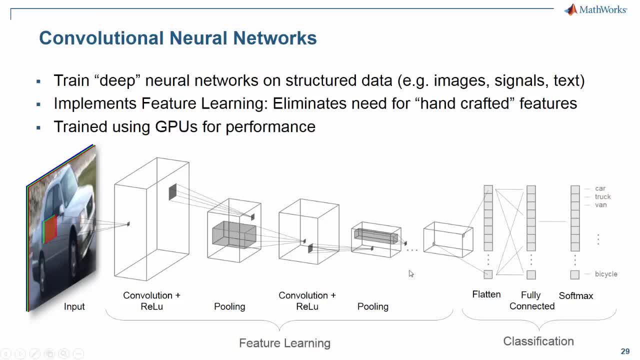 classification stage all these features are put together in some matrix forms, some array form, that, and the label is also available. So in the classification stage there are a number of different sub-stages, like the flattened stage, fully connected stage, softmax stage, as they are. 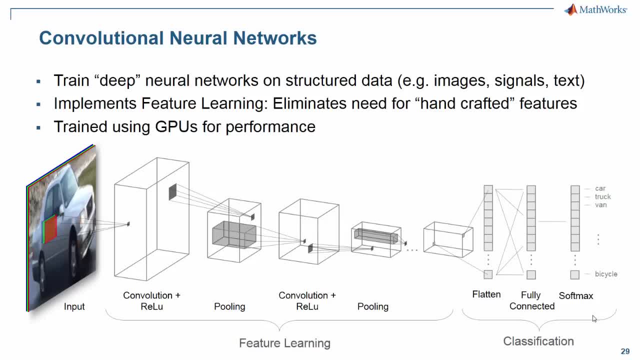 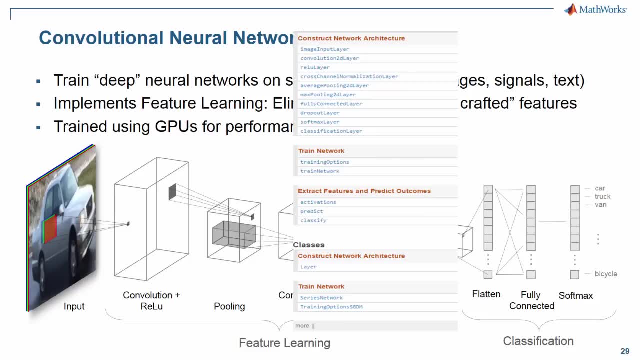 known in the theoretical sense. How can this be helpful? Well, the neural network toolbox. with the deep learning it has got functionalities that tie easily to the theoretical definition. You have got functions to do the convolutional 2D layer, ReLU layer, max pooling layer. 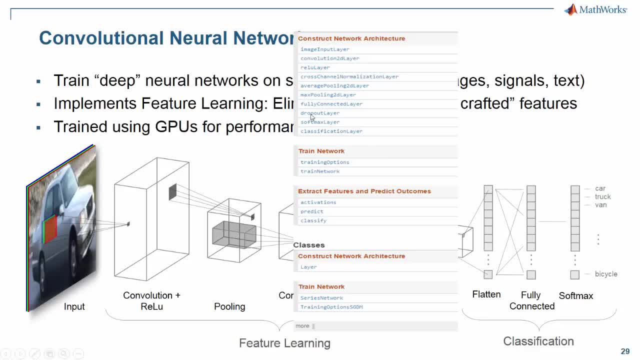 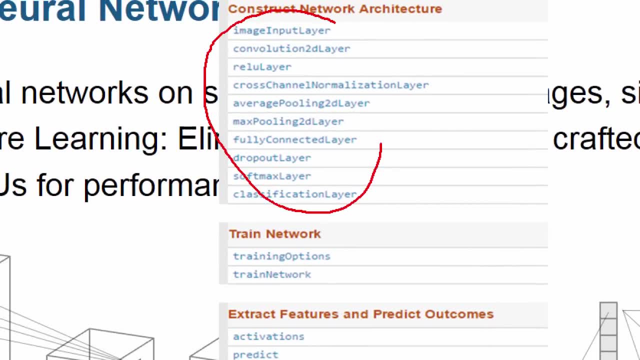 You can build the softmax layer, classification layer, fully connected layer, and so on and so forth. So you have got range of functionalities to construct the architecture That is the deep learning architecture. You have got a range of functions to train the deep learning network. 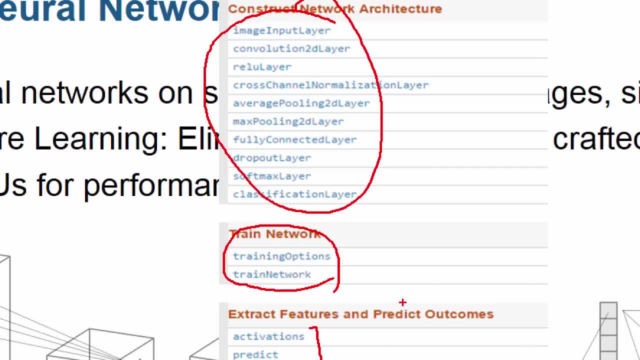 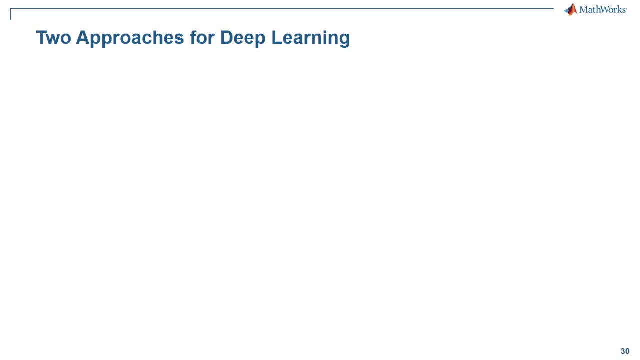 And once the deep learning network is trained, you have functionalities to predict the outcome. You can use the network for prediction or classification, And this is all present in the neural network toolbox. now, Okay, having introduced you to the deep learning network or the convolution neural network, what are the approaches for deep learning? 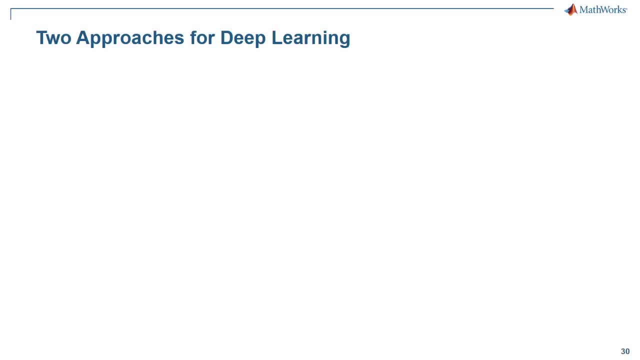 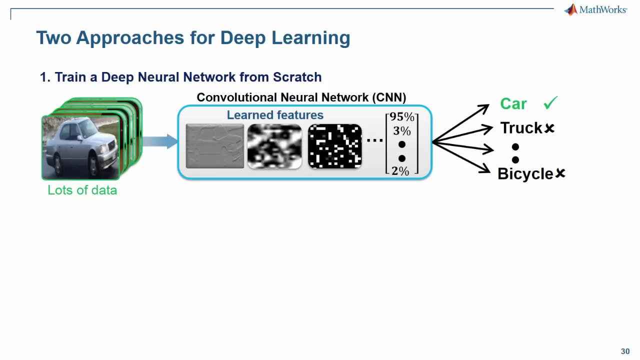 or how can you build a deep learning network in MATAP or how can you make use of all these functionalities which have just been shown to you? There are two approaches. The first approach is to build the deep neural network from scratch. You get in lots of images, maybe you can connect to. 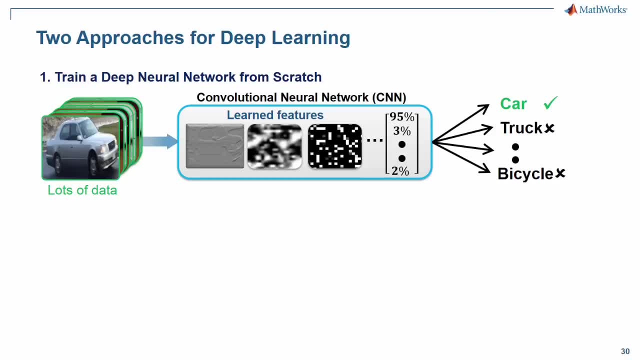 a database, get in those labeled images, push these labeled images through the convolutional neural network, use those functionalities which have been introduced in the convolution neural network toolbox or the neural network toolbox, and then you can design your own architecture and then use that network. 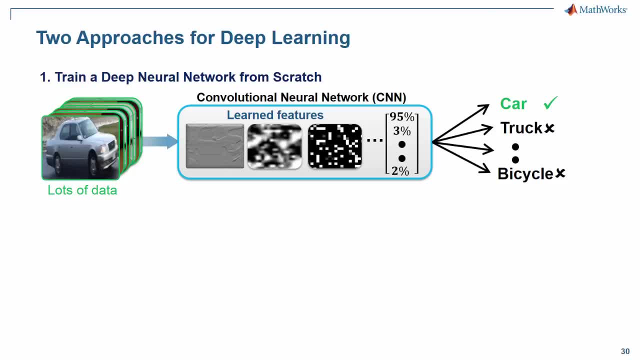 network for classification or prediction. Now, obviously you're starting from scratch. So the first, this particular approach, is going to take time. You can go for a second approach where you can take a pre-trained model and fine tune a pre-trained model for your data. This could be something like performing net surgery. 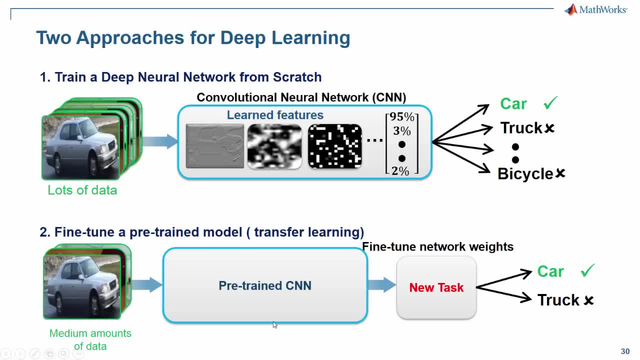 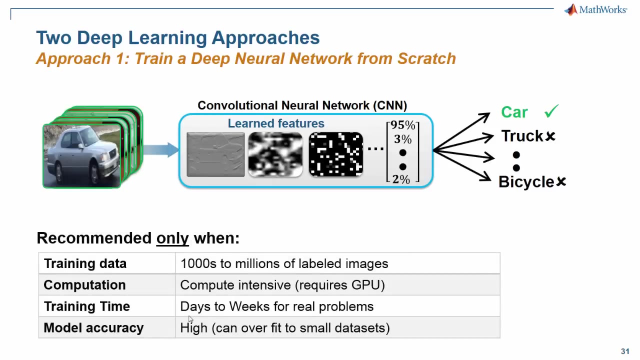 So a particular pre-trained network could be trained to recognize 20 such classes. You want to trim that down to recognize only 3 or 4 such classes, So you can fine tune that particular network. And because it's already been done, you are saving some time over here. So let's try to see the first approach. The first approach trains the. 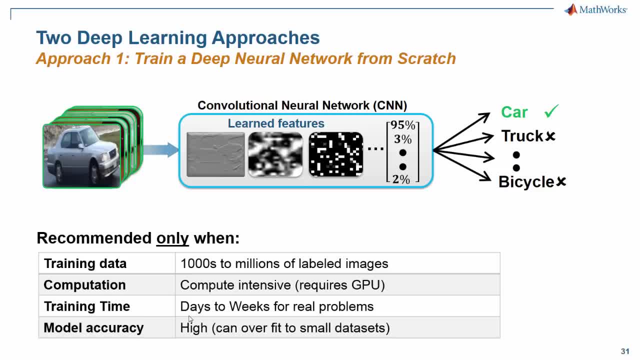 deep neural network from scratch. Now, this is only recommended when you've got lots and lots of other things, so of labeled images also. you want to, because you're playing with lots of images. you need to make sure that you have got access to a gpu, because you'll be all you'll be offloading the computations to. 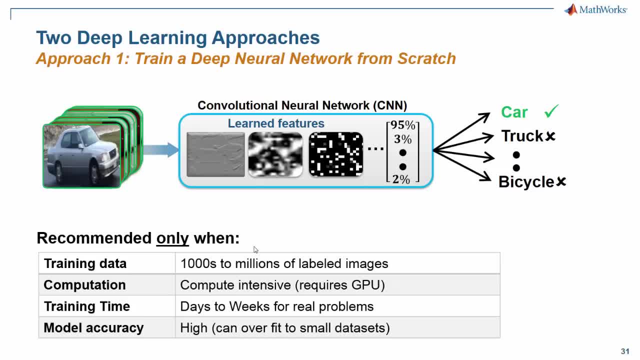 the gpu now because you're dealing, uh, the network from scratch, training the network from scratch. it will take some amount of training time and really days, two weeks, but definitely for lots and lots of images it'll take days, two weeks, but definitely not as long as what we took as a. 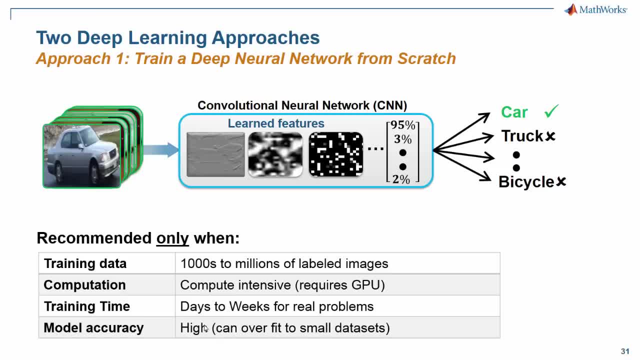 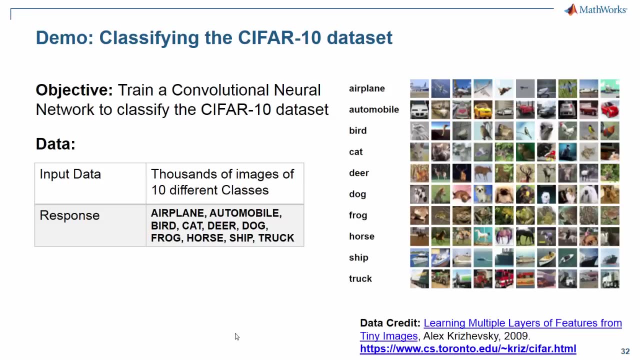 human being to understand the difference between car and suv, not eight or ten years. and because you're dealing from scratch, you're constructing from scratch. the model accuracy in this case is high. so based on that, that's that's our first demo classifying the c far 10 data set. now over here. i. 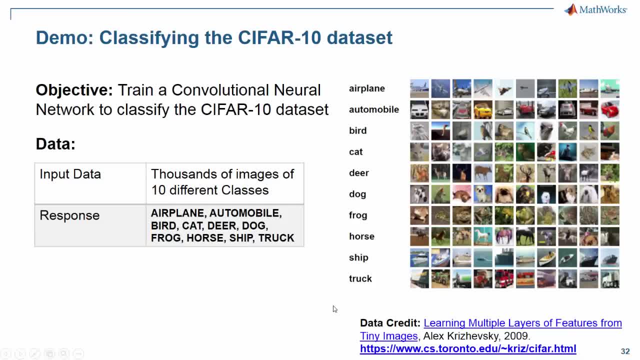 have extracted. i've got this, these images, from our website, and those images are available for 10 different classes: maybe aeroplane, automobile, the different animals, or even a ship or a truck. so there are different 10 classes available. so our job is to design this convolution, neural network, construct this architecture, push. 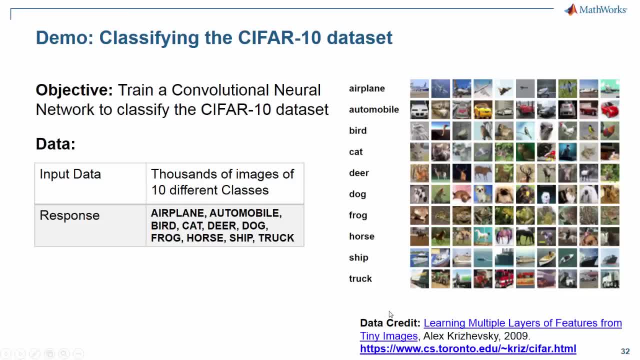 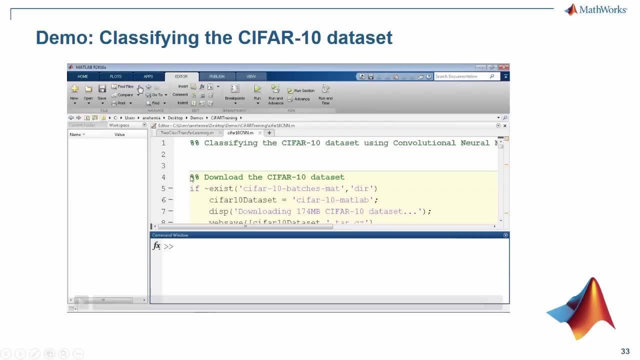 these images through that architecture train, the network and then use the network for classification on a test. okay, so we'll be importing the data defining the architecture train and test the convolution neural network, deep neural network. now, because i don't have um, a gpu, a card on my machine, i won't be able to run it. so what i'm doing over here? i'm presenting you a video. 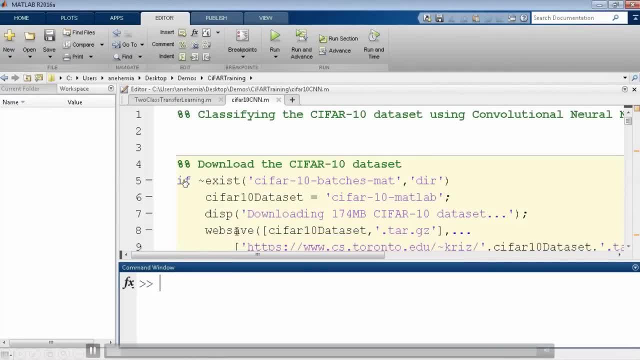 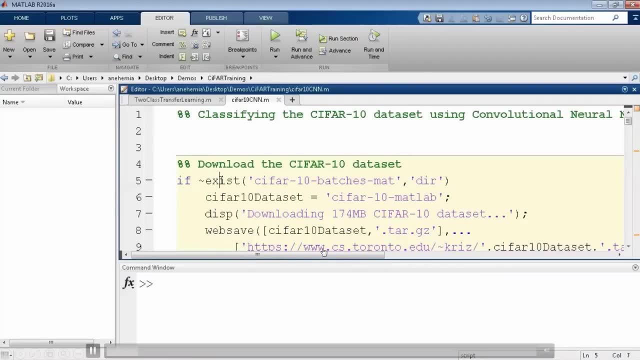 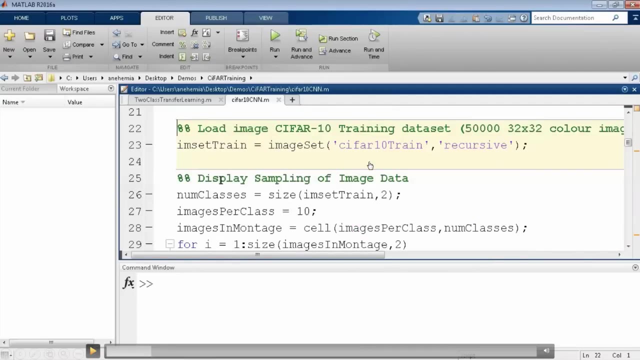 for that same c far 10 data set. now over here in the first section, we'll check whether the data set is present inside your computer. if it's not, matlab can also connect to that particular website to download that particular data set. now, when that particular data set is downloaded, it will be. 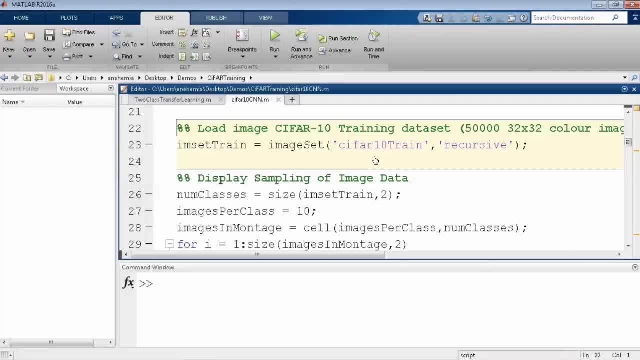 present in different folders: a folder of images for automobile, a folder of images for deer, a folder of images for ship and so on and so forth. now you want to access those images, so you want to go for the recursive fashion. so you'll be making use of image set image. that is pretty much. 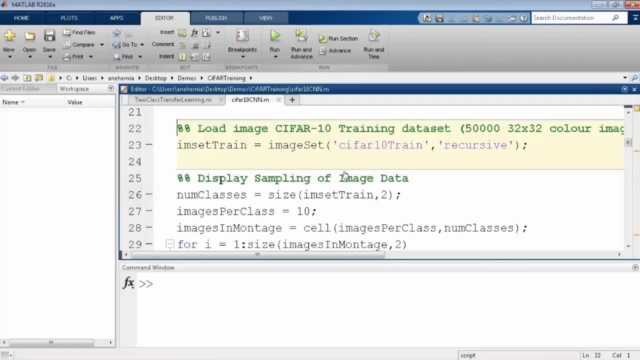 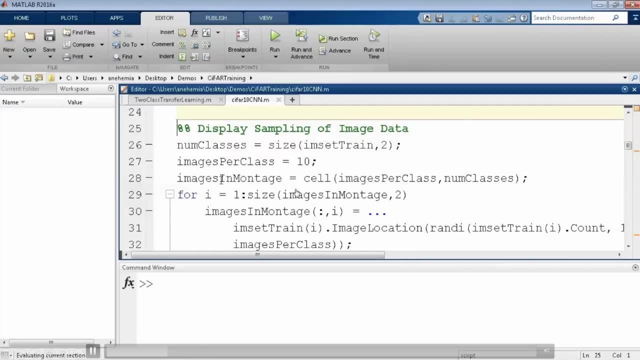 used when you're playing with large data set, large image data set, another recursive form. after you finish playing with images in the first folder, go to the second one, and so on and so forth. so that's what it is doing over here: accessing those images and then in the next set. i'm just 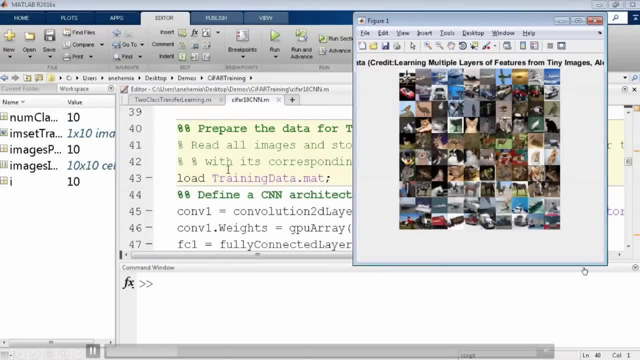 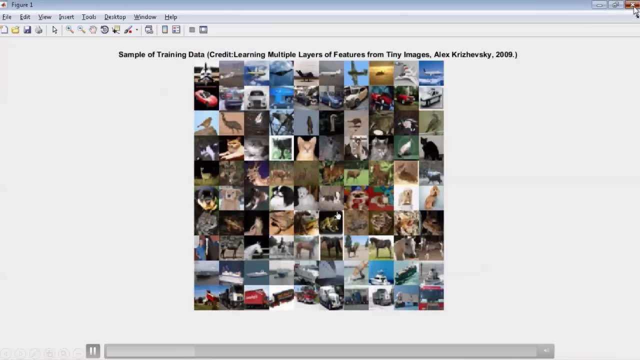 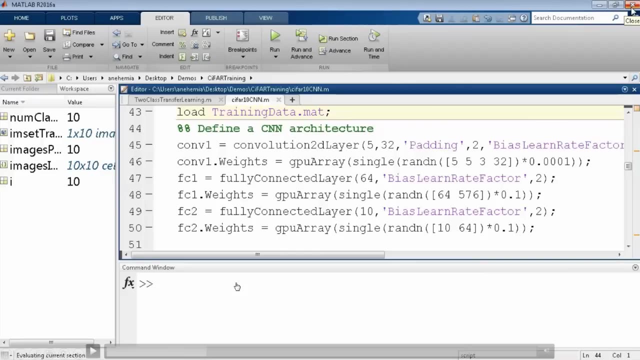 uh, displaying a sample of image data, maybe 10.. i want to just check how it looks like, right? so this is just a sample. this is some one touch of those images. once that is done, i'm moving forward to load the training data now with those images i had. i've already divided. 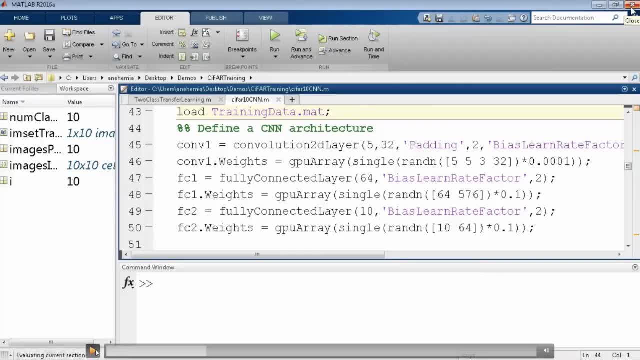 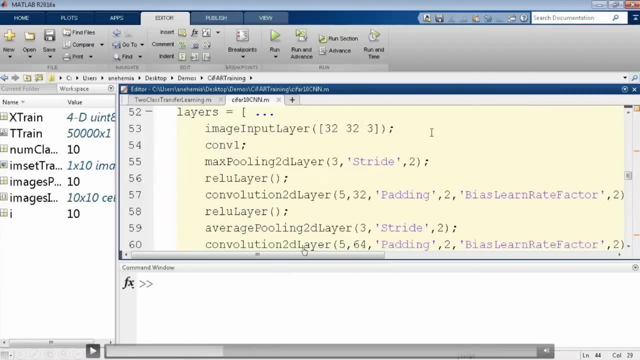 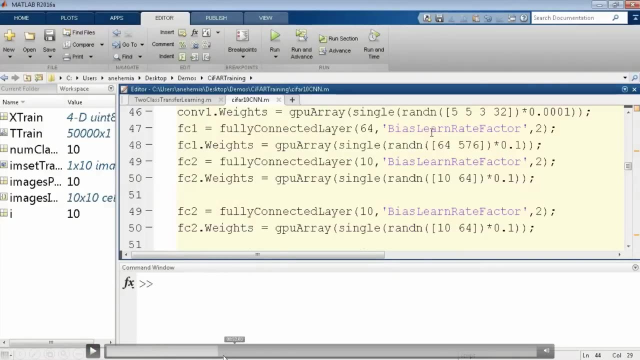 into a training set and a testing set and it's present in the respective mat file. so i'm just loading in the training data set and what's coming up next is the approach or is the construction of the architecture. so over here, if i just go back, you could see that i'm trying to construct, define. 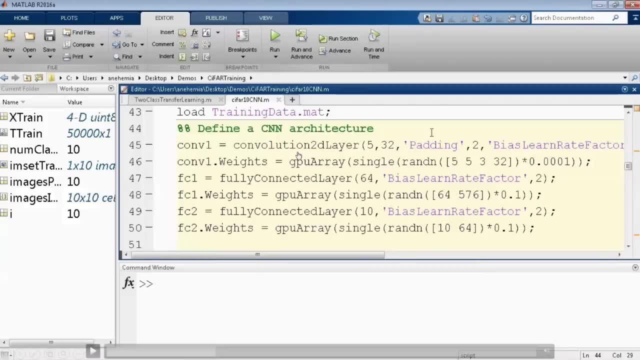 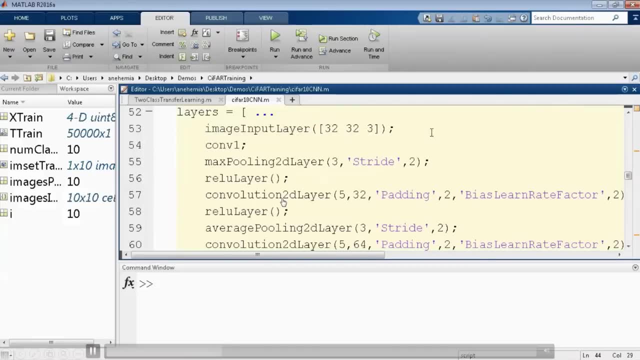 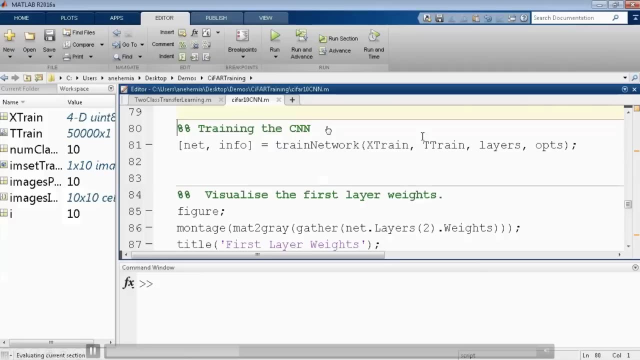 a cnn architecture with convolution 2d layer, fully connected layer and after each thing, i'm just trying to move those variables from the gpu because the computations will be taken on the gpu. i'm not defining the layers: average pooling layer, regular classification layer, putting all those settings and once the network is defined, i'm using the train network. 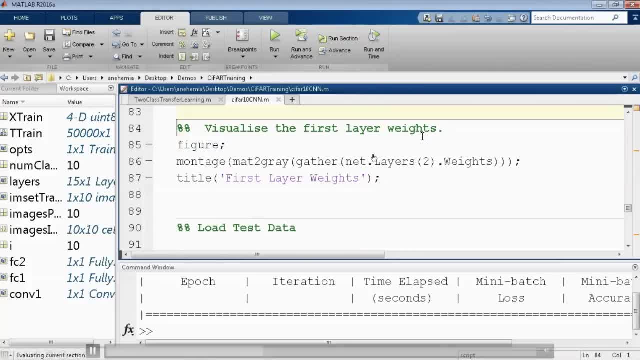 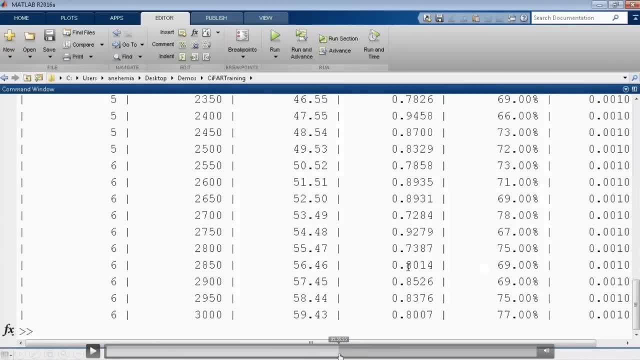 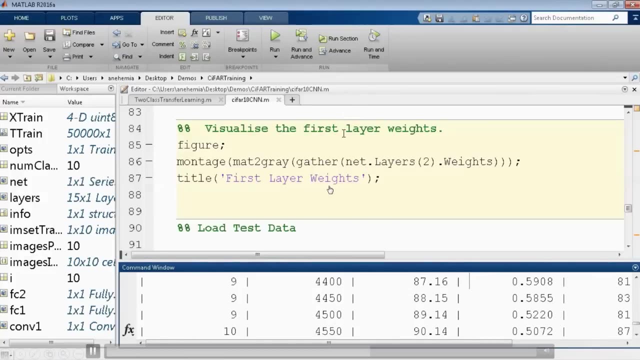 function to train the data set and then it spits out some results. how long it has taken to train? typically it's taken about 5000 iterations to come up with some results. once i'm done with that, i'm just wanting to see how the layer, how the first layer, weights look like, and this is just an image plot. 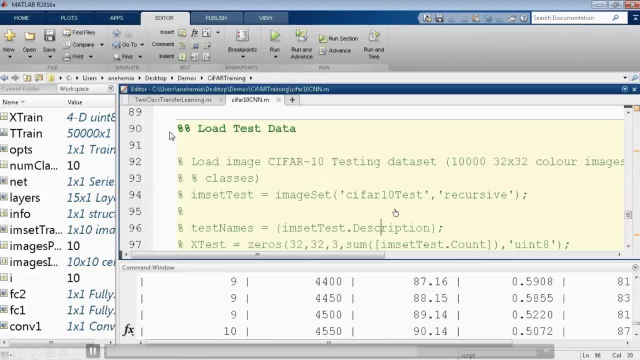 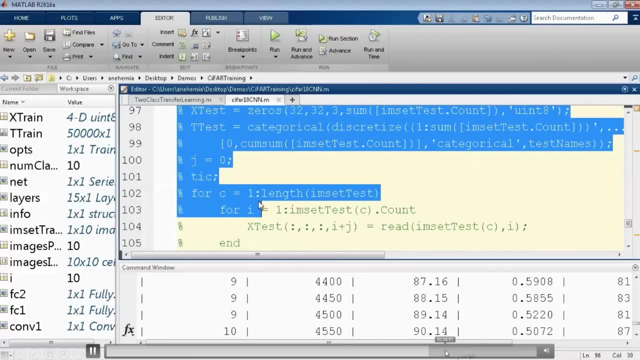 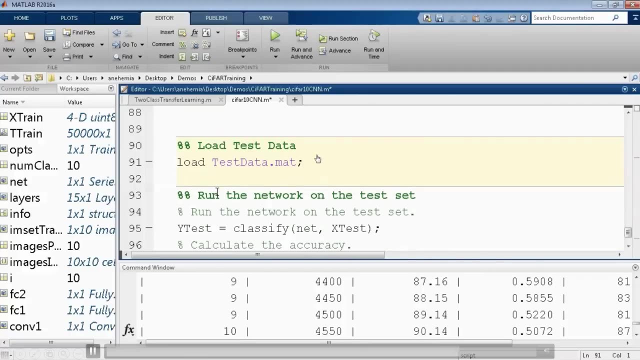 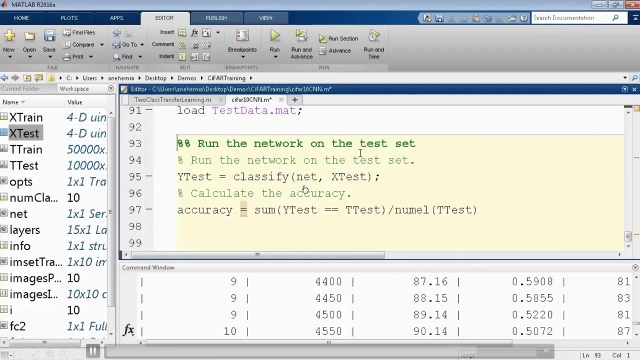 of the first layer, weight. once that is done, i'm trying to load the test data set. so i'm just making a few changes over here. i'm just trying to get rid of those comments and load the test data file. so i'm just loading it that, and once that test data file is loaded, i want to use the network which i 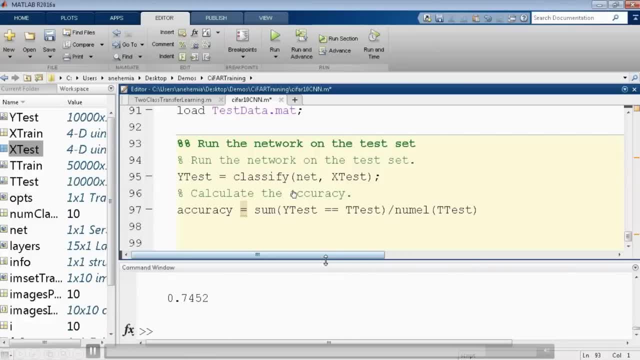 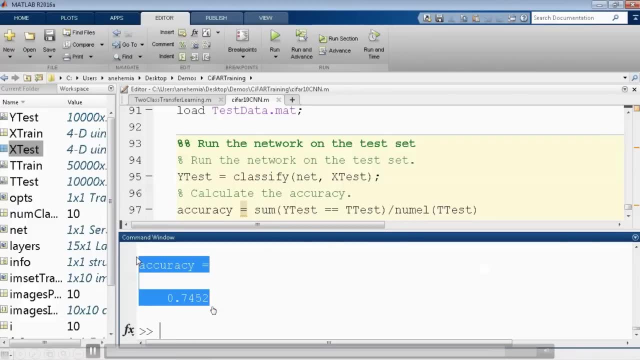 just built and trained for classification purposes, and it also spits up some accuracy. i want to check what the accuracy is over here. the accuracy is about 75, but if you had some more layers added, some more, if you had an extensive architecture, you can again play with this accuracy as you need. 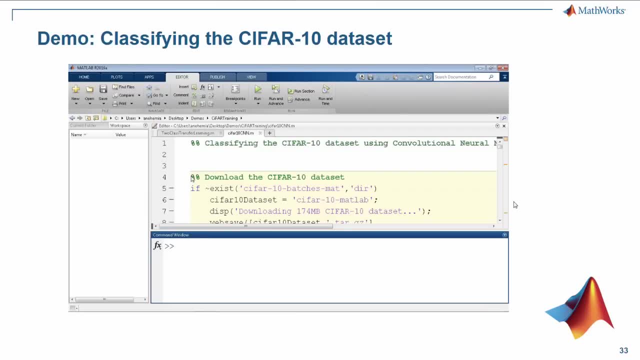 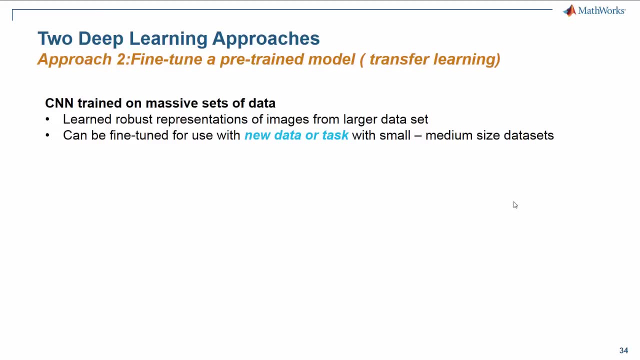 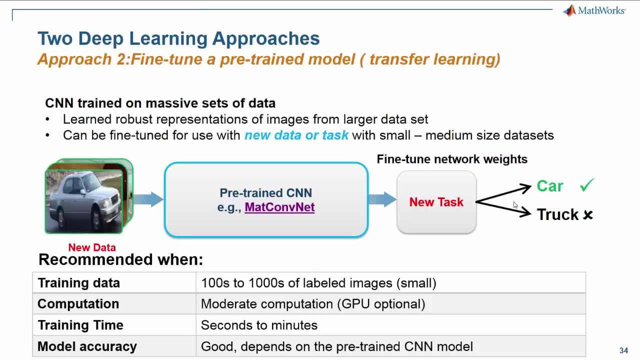 okay, having seen how to construct this deep learning network, the second approach over here we have is how to use an existing deep learning network and fine tune it now, especially when you have lots and lots of data and you have very little time to construct that network. you can use an existing network from a website. 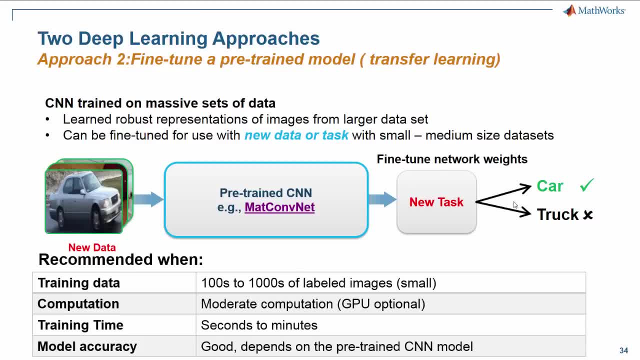 and do some net surgery on it and use that network for your application, for your data set. so especially use. when the train data set is small, moderate amount of computation is required. training time is very quick and model accuracy is good because you're using already pre-trained network and you're changing a little bit in it. 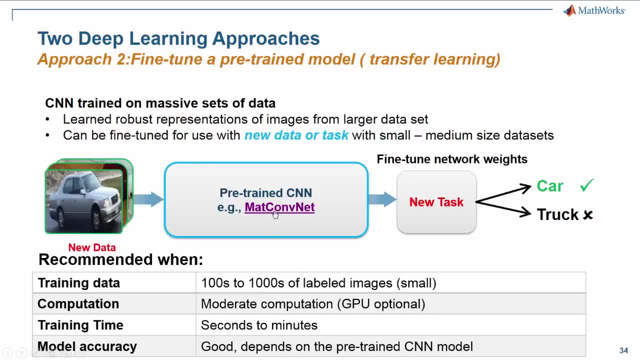 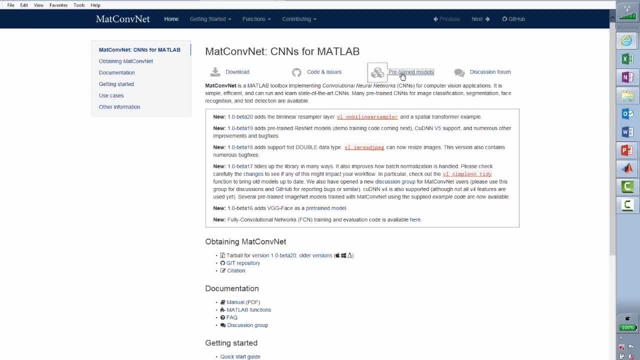 now, where can i get these pre-trained models? there's a website called as matconf net so we can visit that website and over here in that matcon net there is a section for pre-trained models, pre-train models in matlab. so you've got free train models for face recognition segment. 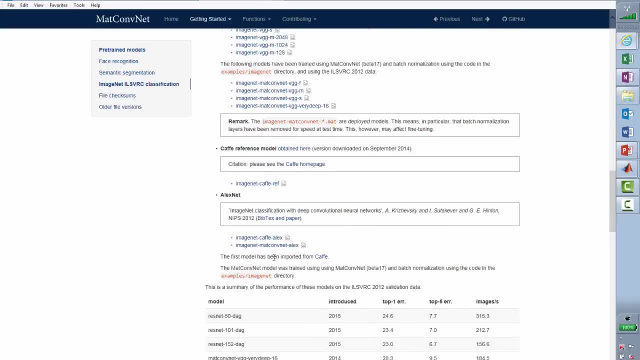 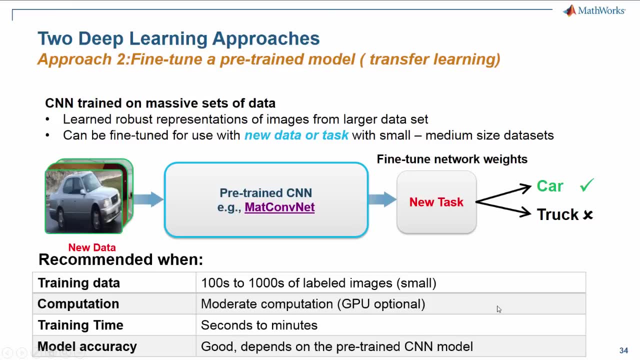 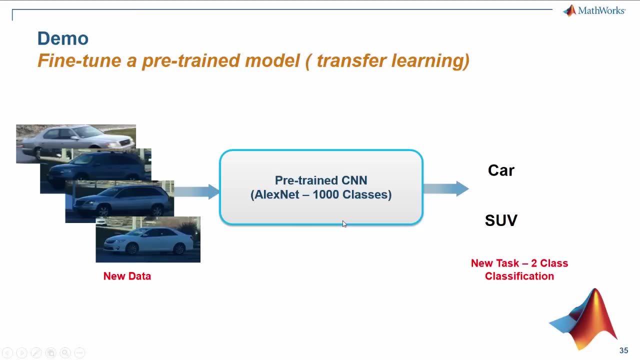 x segmentation, image net classification and so on and so forth. so one such model has been used in our next demonstration and that is called as alexnet. so over here you have. we've used some existing pre-trained model, alexnet from that point of view, that is, the pre-trained models over here. 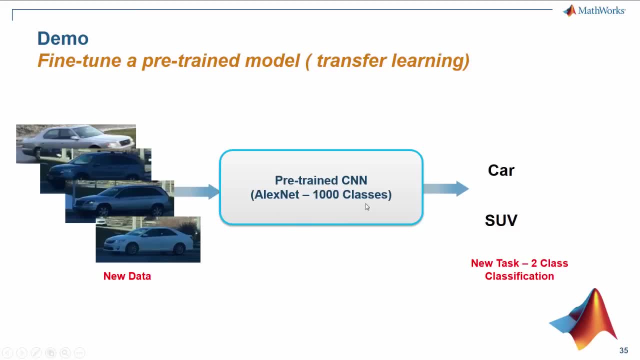 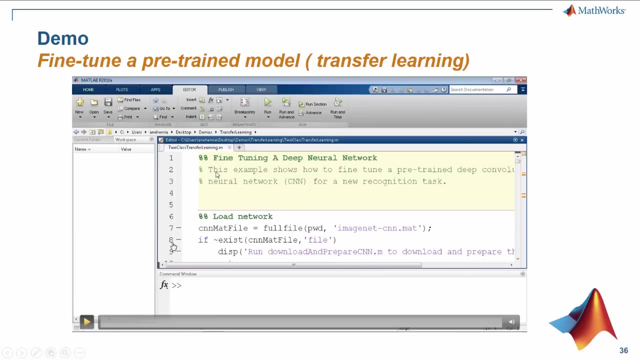 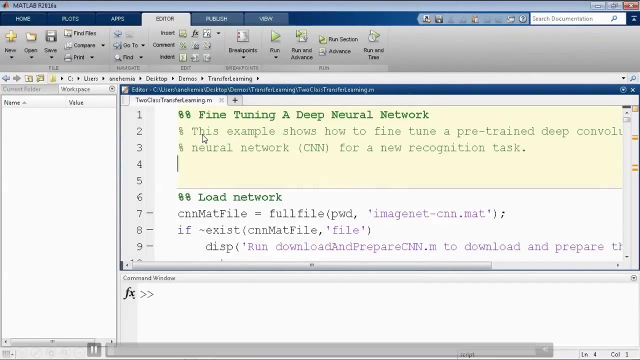 particular website, matconnet, pushing in our data set, tuning that, our tuning that existing model and and using that for classification. the interest of time. we won't be, unfortunately, going through how this model works, but there is a video over here in place if you were to look into it. so we are loading in the network. 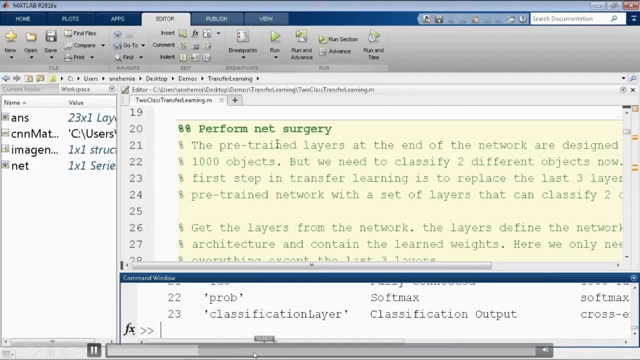 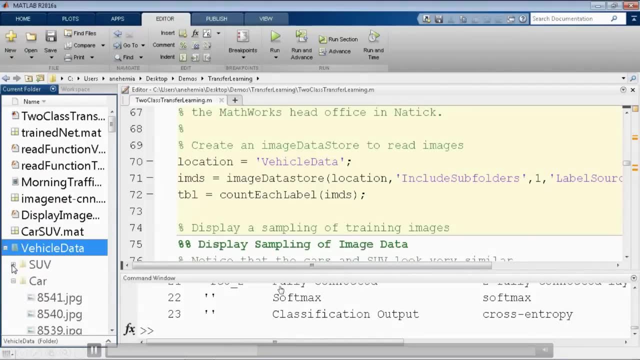 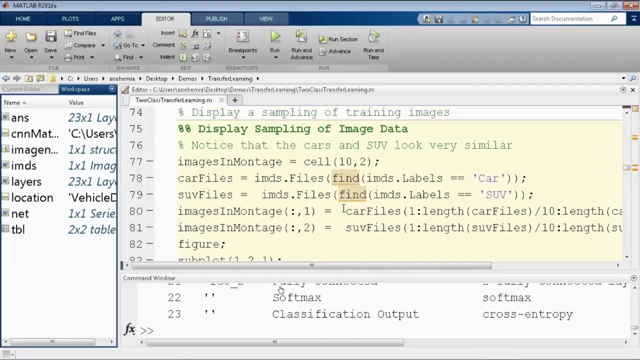 then we're performing some net surgery, adding in some models, adding some extra layers, and then we are using that network for classification purposes. so you'll be having a look, you'll be getting these slides and have a look at that particular video and see how things could be altered to suit to your data. 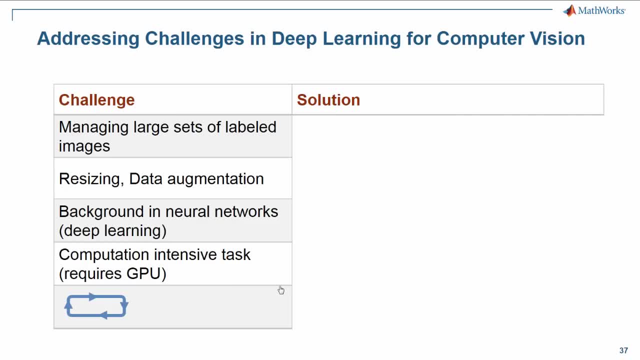 set. so the challenges which we saw: managing large sets of label data. let's have a look at how can we address these challenges. so image net or image image set or image data store: is that particular functionality available if you want to handle large set of images, if you want to resize or do some pre-processing on your? 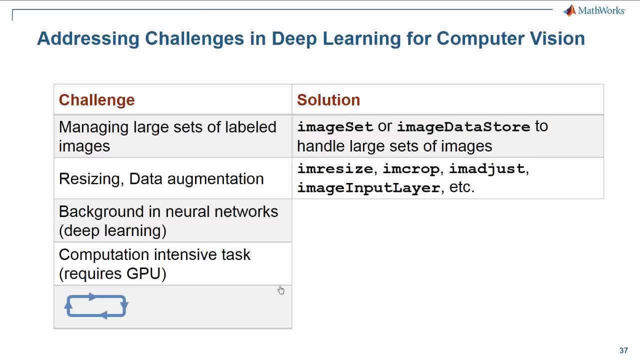 images that are supporting functions, part of the image processing toolbox. functions like I am resize, I am croc, I am adjust, and so on. they could be useful if you want to do some pre-processing, do you want to have a? if you have a background in neural networks and if you can want to construct your own, a deep 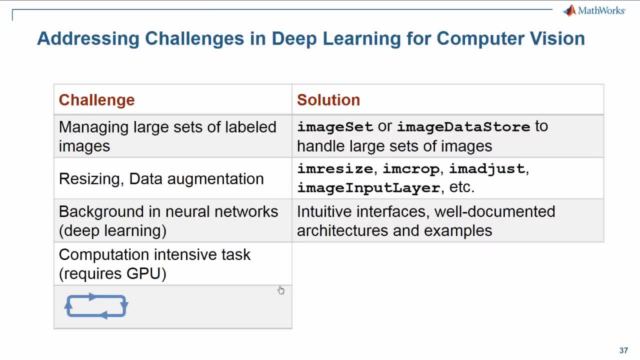 learning network, then we've got this neural network toolbox. it has got all these functionalities suited if you want to have your own deep learning network to be constructed. at the moment, all these functionalities which we have seen, the training needs to be supported on GPUs and as and there's this function, GPU array, which can help. 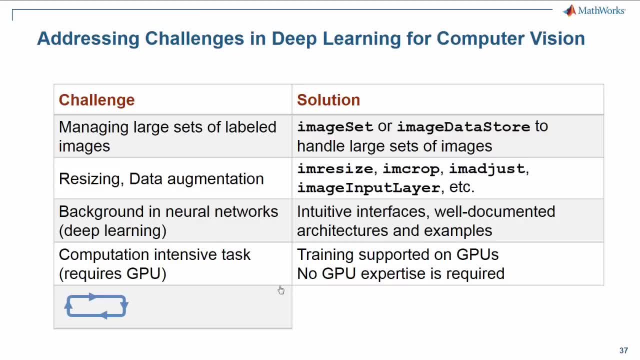 you translate the variables from your own MATLAB to the GPU. so, and there's no GPU expertise required for this. and, of course, because it's MATLAB, it's not a GPU, so there's no GPU expertise required for this. and, of course, because it's MATLAB. so, and there's no GPU expertise required for this, and, of course, because it's.